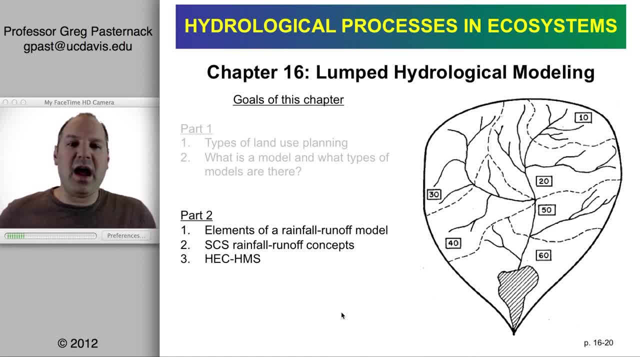 This is the part two video podcast for chapter 16 on lumped hydrological modeling. So in the first part I covered just the general idea of modeling and the different kinds of models. Now we want to get right into hydrological modeling In the long run in this whole section. 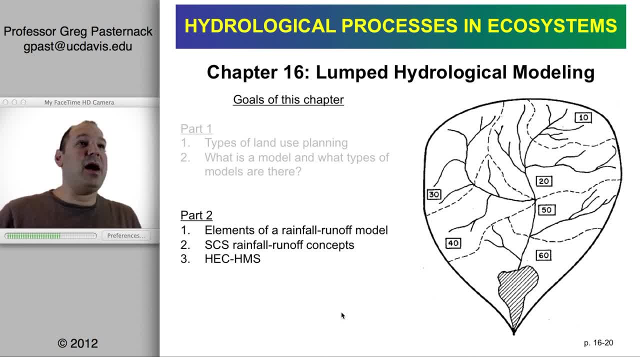 for the rest of the course. here we want to get into fairly complicated models that are going to deal with ecology and a variety of applications of hydrology and eco-hydrology, But for right now we want to start with the most essential basics. How can we take rainfall and turn it into runoff? 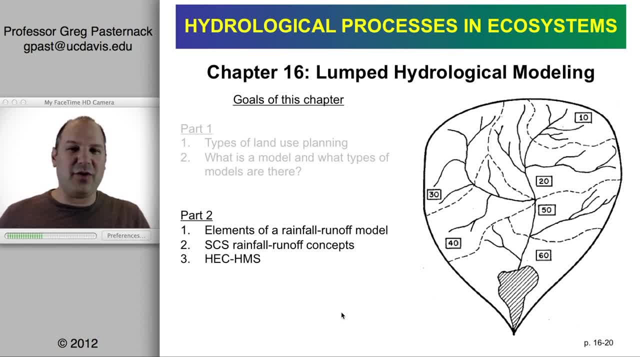 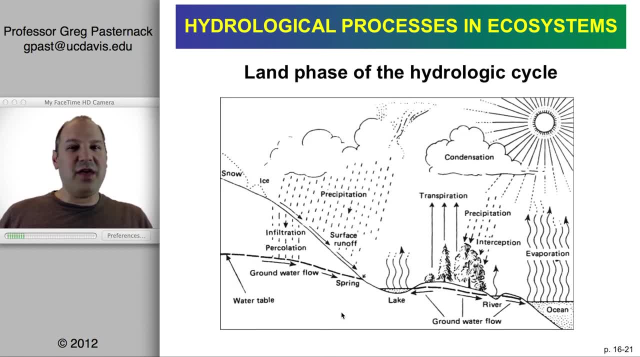 If you can do that, then you can pretty much do professional hydrology as an entry-level hydrologist. And of course, a hydrological model is going to start with the hydrological cycle and compute the elements of the water balance, with a special eye towards calculating runoff. 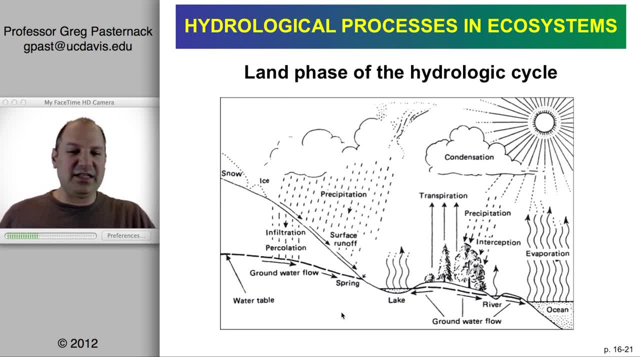 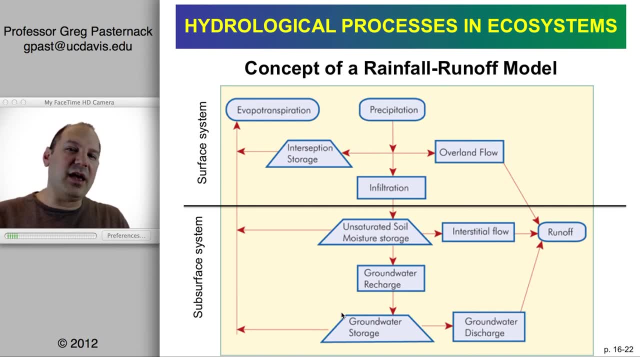 There shouldn't be any surprise in the processes that you see on this slide. Just a reminder of what we're doing here. So what we do is we take that graphic and we turn it into a flowchart schematic. In this flowchart we try to list all of the individual stores and processes that are taking. 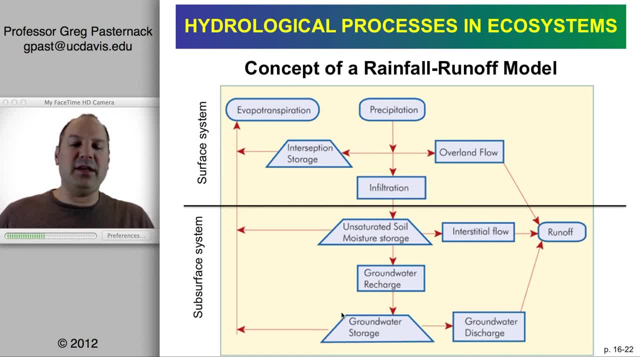 place. So we have water stored as precipitation or evapotranspiration, and then it's going to flux from one to the other. Some of these are more fluxes, some of them are more stores, But the key is that we need to characterize all of the processes that are taking place. 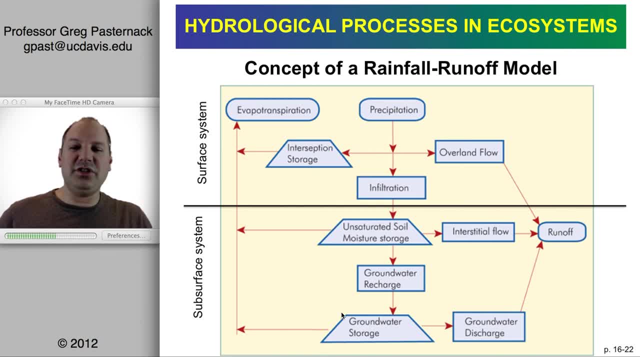 And then we just have to make interesting and challenging decisions about how much detail to represent each process. You could also see that this schematic breaks the land into the surface system and subsurface system. Obviously, water flows across the land surface boundary seamlessly, but still it's very convenient to break the processes up this way, And the vast majority 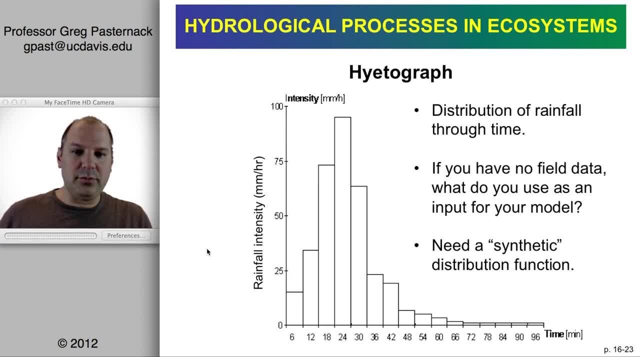 of models that are used do that Okay. so the first process is obviously precipitation, And we can represent precipitation with something called a hiatograph. Just as a hydrograph presents the change in discharge through time, a hiatograph represents the change in precipitation through time, In this case showing it in terms of rainfall. 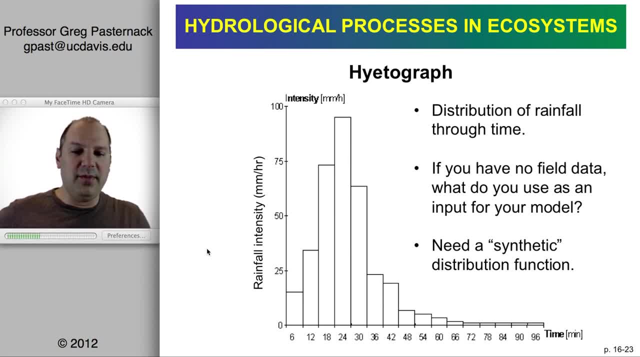 but it doesn't necessarily have to be rainfall, And this is just your typical histogram of the amount of rain, discretized into minutes in this case. Now, obviously, you can't make a hydrological model if you don't have a hydrograph, So what we're going to do is we're going to take a 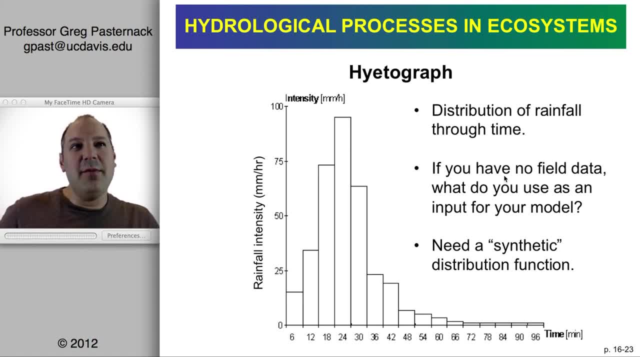 hydrograph and we're going to start with rainfall and turn it into runoff. But of course, the majority of uses of hydrological models is not to model some past event but to conduct planning to figure out what would happen in different idealistic scenarios. So, for example, you could: 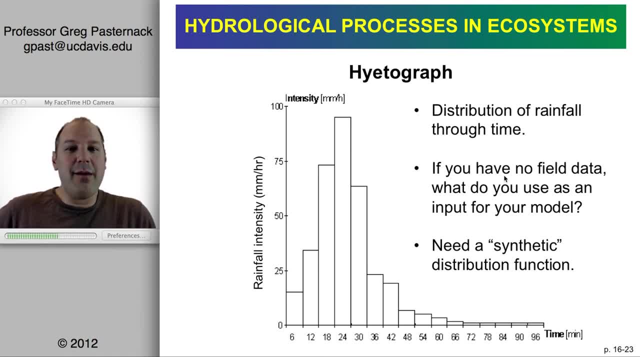 say: well, I'm worried about the hundred-year flood. Well, how much rain do I need to represent that flood And how do I distribute that rain through time? So, as a result, we need a synthetic distribution function that's going to represent the hydrograph through time. It's easy to specify. 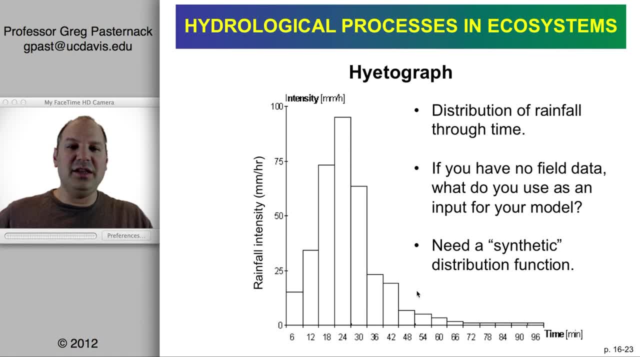 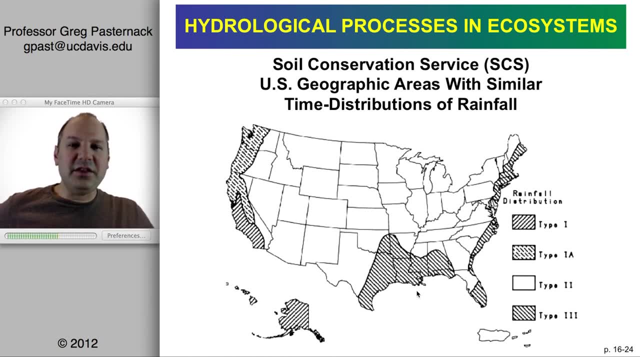 an amount, but how do you specify that pattern? This is like the rainfall equivalent of the natural flow regime on an event basis. Well, for a lot of the things I'm going to show you in this video podcast, government scientists have done a lot of work all over the United. 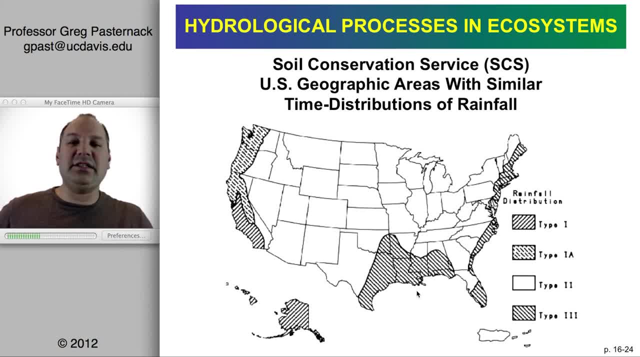 States to try to figure out how the processes vary geographically. This is a relatively simple, crude schematic that shows what was figured out: That basically across the United States there are four different types of rainfall distributions through time And you can see the vast majority of the United States falls into a type two category where we are in the Central. 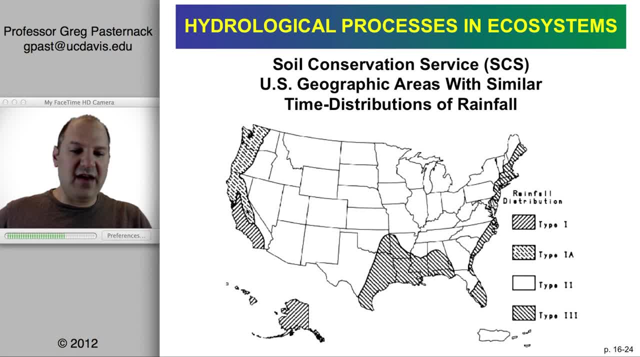 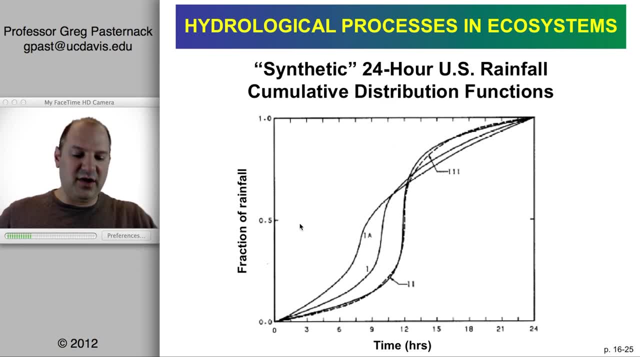 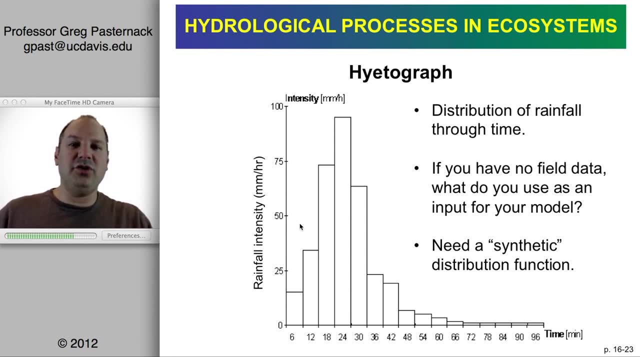 Valley falls into a type one and the Sierras have a type 1a. So what does that mean? Well, this shows the cumulative distribution function. So remember, like the histogram is what we call a probability density function, So it just shows the incremental. 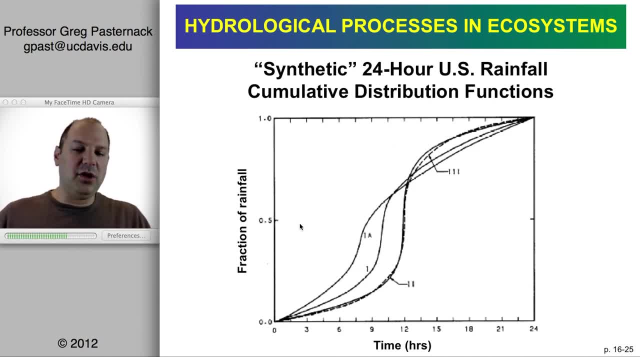 change through time, whereas the CDF shows a cumulative amount of water through time. So in Excel you should be able to work pretty interchangeably if you have a histogram to convert. you know, sum up the numbers to get the cumulative numbers, or subtract one from. 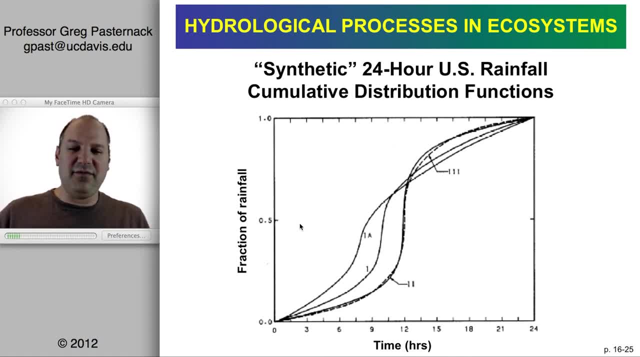 the next to get the probability density function And so this shows the fraction of rainfall through time. So you can see that like a type two event is, you know, has a relatively slow increase in rainfall, then a huge amount of rainfall in a very short time and then a you know. 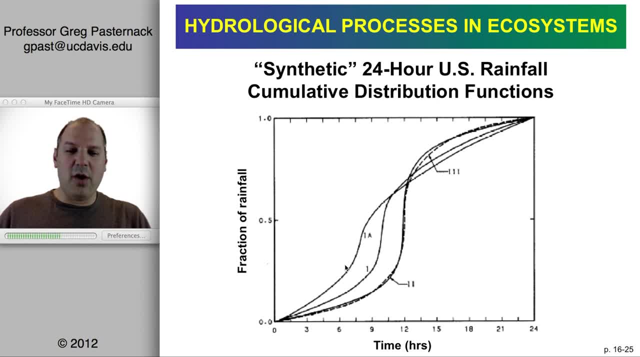 a small amount of rainfall again. whereas, like type one and 1a are more gradual storms, they still have a peak, but it's just not as extreme as what you see in the type two and type three events. right, Yeah, Okay. 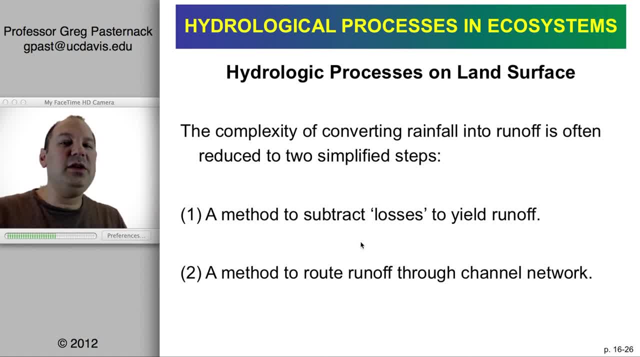 So that's the rainfall. So now we're going to talk about the rainfall and how we're going to handle this, And you will be doing this in assignments, So it's important to you know, have a basic understanding before you actually get into the thick of it. So now you take your rainfall and you 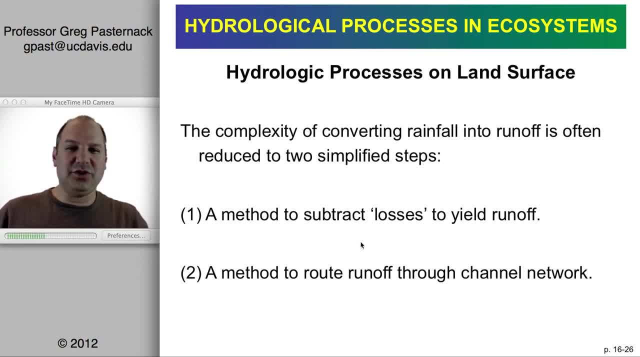 want to remove water as a result of the losses that take place on the land. We've talked about a lot of those different kinds of losses already, So how do we put that into a model, And that's what I'm going to show you? So we're going to consider different kinds of 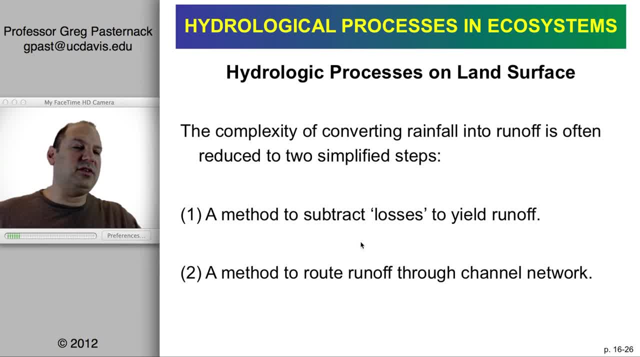 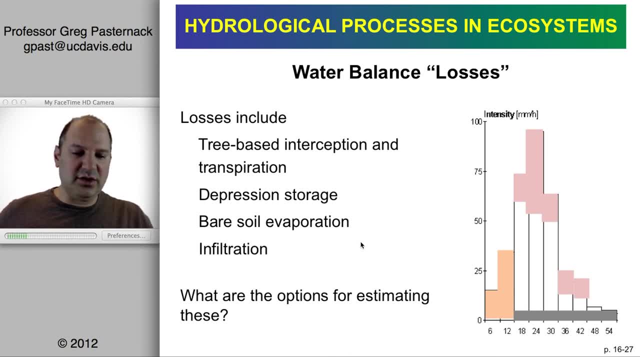 losses. So if you've removed the losses, then you have to take the excess water that runs off and then route it through the channel network. So how do we handle losses? So if we take the precipitation through time, which I've shown here again, the X axis is time, Y axis: 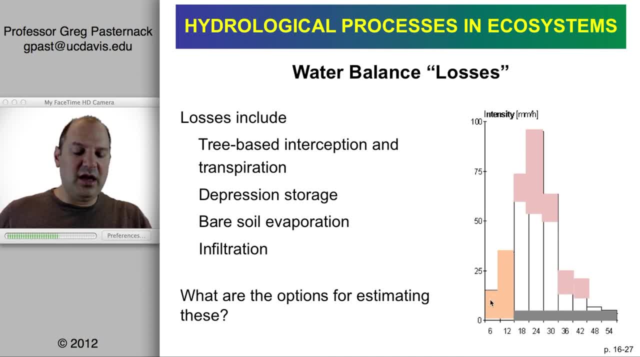 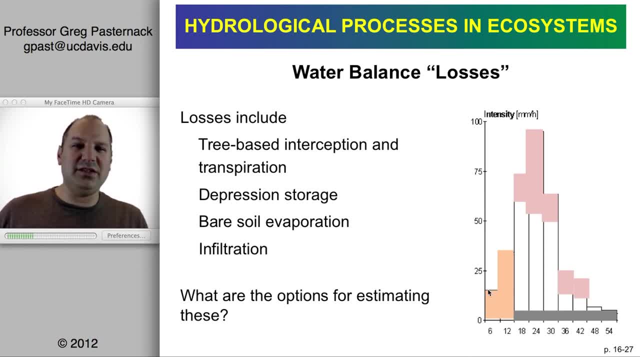 Okay, So in the initial instance when rain begins, water is going to be stored and it's going to store, store, store until eventually you have enough run off. I'm sorry You have enough rainfall to overwhelm that storage capacity and have saturation. 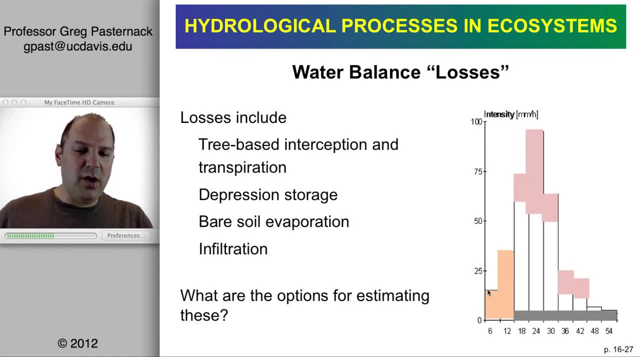 excess. Okay, And so that's going to yield what what is called the initial abstraction, And it's shown here in orange like these two. you know, the first 12 hours, or whatever in this case um, of rainfall. 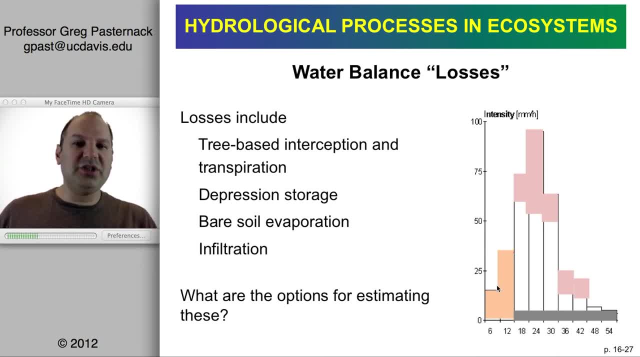 Okay, are all consumed by the watershed, you know like nothing runs off After that. then I've got two different components to losses. I have a constant value that might represent, like tree interception, transpiration might be constant and, you know, possibly depression storage, but yeah, probably. 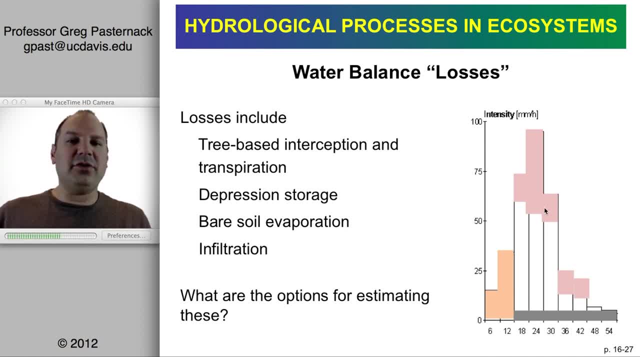 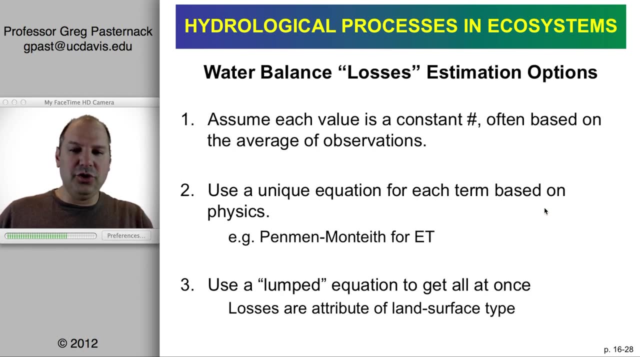 not. And then I've got the pink component here, where the amount of storage changes through time, and that could be soil storage and it could also be depression storage, because that can grow as different areas of depression are, you know, filled up. So what we're going to do, 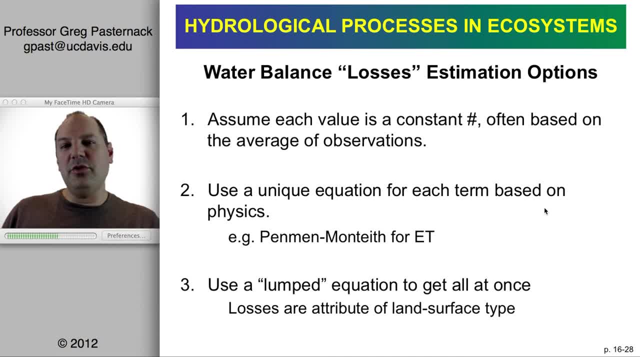 is we're going to look at different ways of doing it and then go through the most common way that's used, you know, in a lot of the consulting world. The first thing is you could assume each of these terms are constants, but that's a relatively poor choice. Another thing you could 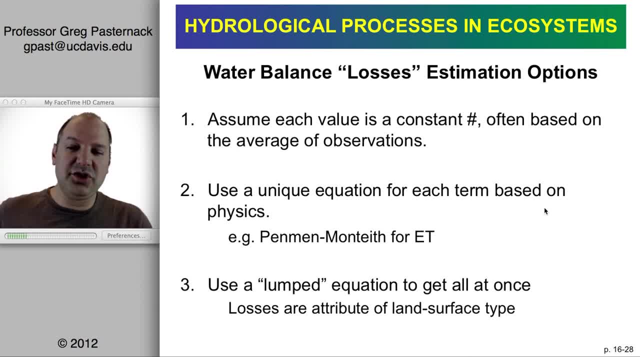 do is you could get a very complex equation and you could get a very complex equation for each term, Maybe go out in the field and calibrate it for your site and then apply those- and certainly there are models that do that. But a more common approach is to do a lumped approach. 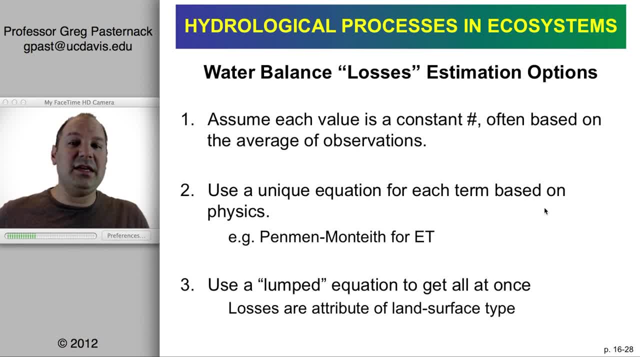 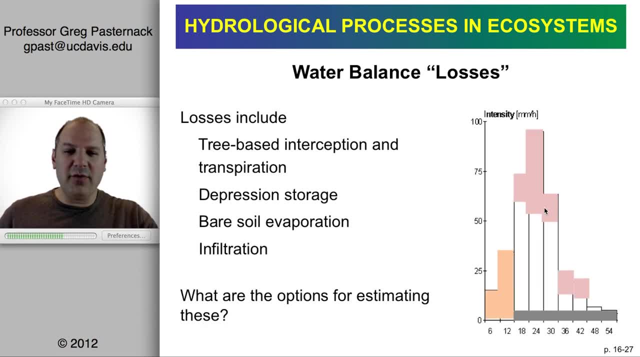 So, in the same way that we can treat the whole watershed as one entity and talk about that being a lumped watershed model, we can also lump the processes. So we take all the processes that remove water and lump them all together into one representative. 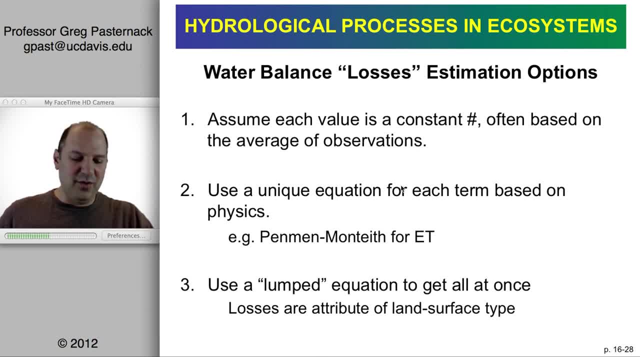 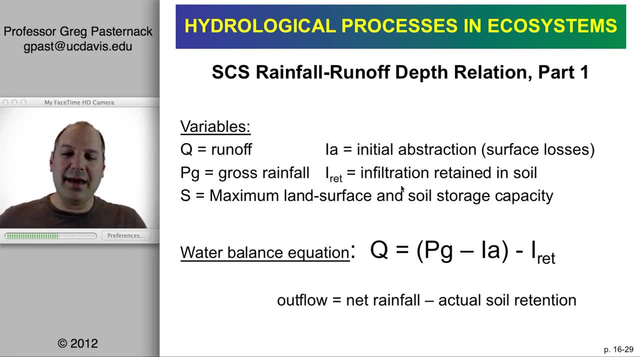 And then the representative process- we just call it loss- then we can do that. So what I want to show you next are some simple equations that are very conceptual, that can be employed to create a hydrological model that does this removal of losses. Of course, we're going to begin with the water balance. right, I mean, you gotta have a water balance if you're doing a hydrological model. It's a basic law of mass conservation. So here I've written: 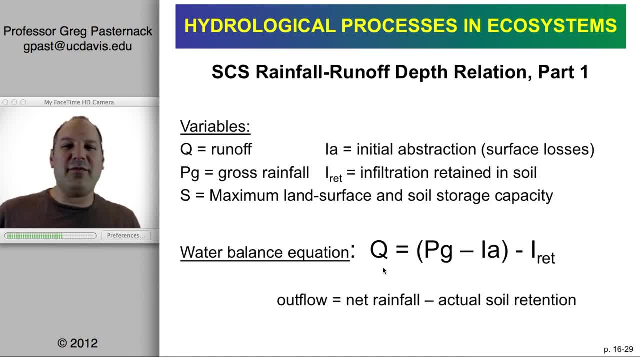 the water balance. instead of like inflows, equal outflows plus storage, I'm just solving it in terms of the runoff or stream discharge Q, And it's going to equal the gross precipitation minus the initial abstraction, minus water that is retained in the soil after the initial. 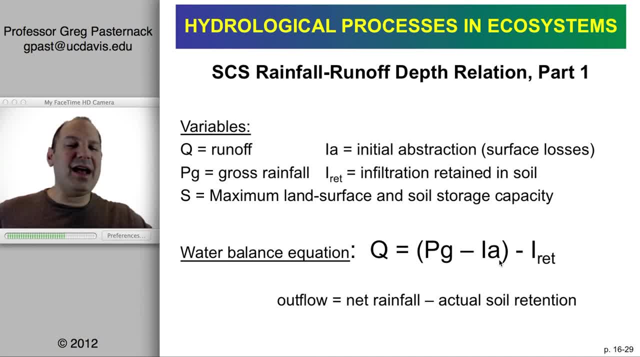 abstraction period. So initial abstraction that's lots of things lumped together And even the infiltration retained in the soil it still could be a lot of different specific stores that are holding that water. So here's a water balance equation. Now we can't just solve this equation. 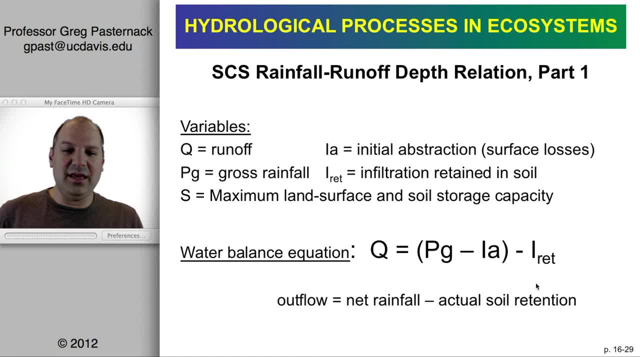 without some mechanistic aid. Ideally you'd want to have a momentum equation. You take mass and momentum together and you can solve that system. However, that's a relatively complicated model to solve. So usually you have to either simplify the momentum equation down or you have to substitute some kind of 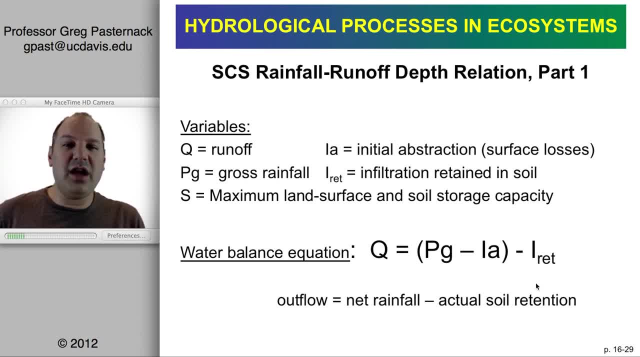 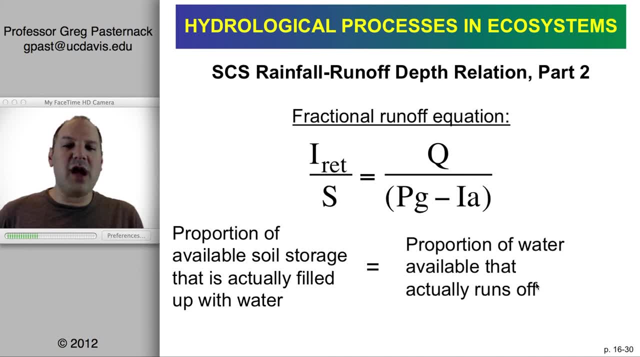 concept, or what we could call a rule that's going to govern flow or storage in some way, And so what happens is that there's a method called the Soil Conservation Service- Rainfall Runoff Depth Relation that provides the key ingredient we need to complete this model. What we do is we say that the amount of water that runs off, 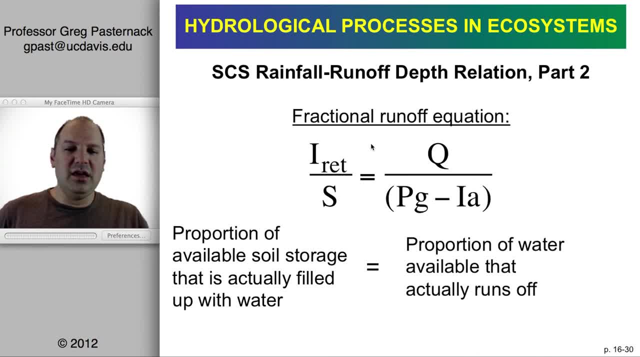 is proportionally similar to the amount of water that's retained as a function of total storage. So on the left side we look at the fraction, the amount of water that's actually stored compared to the total storage, and the amount of water that runs off compared to the actual amount that runs off compared to the total water. 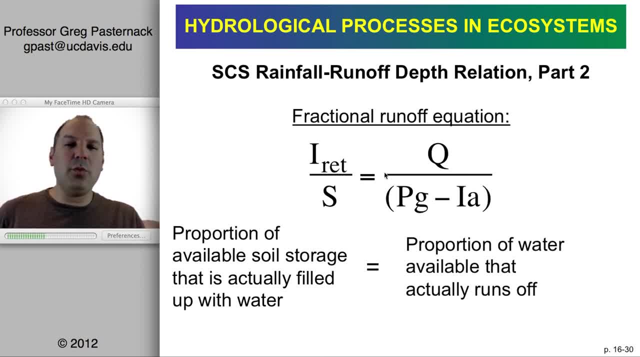 available to run off. So the idea here is that these would remain proportional. So this is a linear transport law. Essentially, that tells us how runoff would function Without going any further. let's just try to understand this, because there's just no way that, you know, we just pull this out of a hat. It doesn't, can't possibly make any sense, But let's just play. 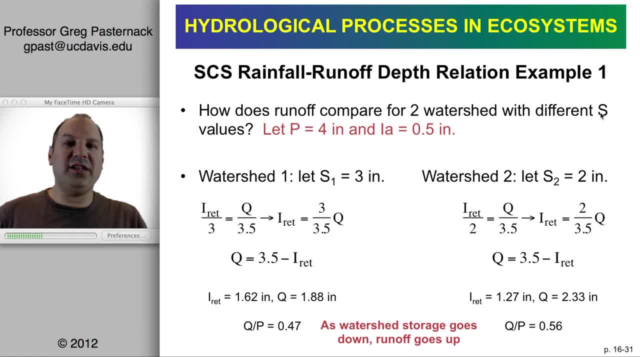 with some numbers. Okay, so let's look at two different watersheds with different storage capacity. So in this case s is total storage of water that we can have. So let's have a rainfall of four inches in this storm and let's have an initial abstraction of half an inch. So if we go to the mass balance equation, 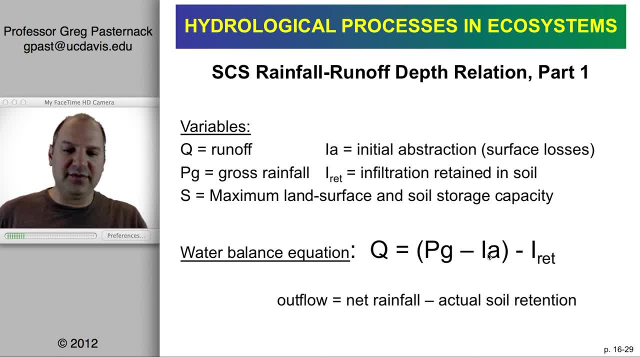 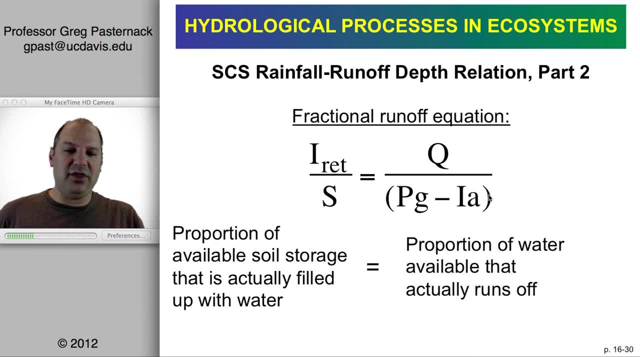 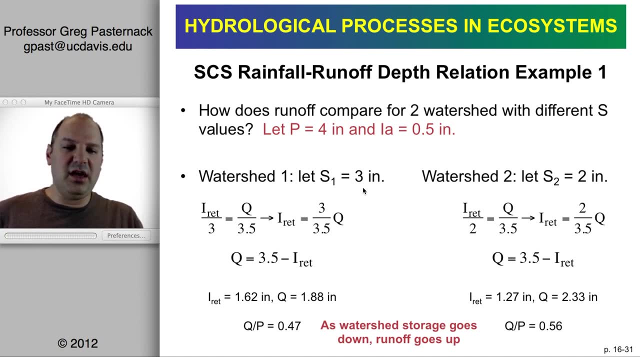 you know, four minus 0.5 equals 3.5.. So the runoff is going to equal 3.5, minus the infiltration that's retained, And then we can similarly put in 3.5 down here. Okay, now let's have one watershed with a storage of three inches. That's the maximum capacity of. 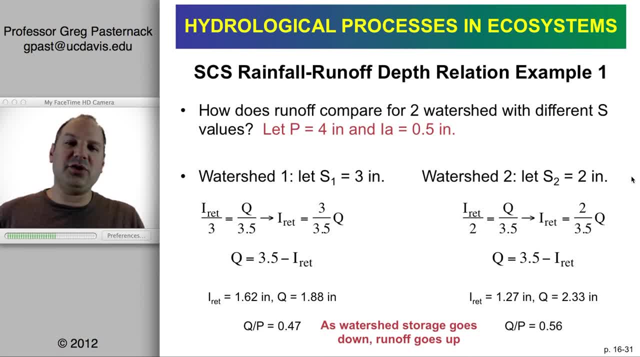 water that the soil can hold and have a sapling, and then one watershed with another watershed with a storage capacity of two inches. If we put the numbers in, we have two equations. So the first equation on the right simplifies- to this here, I'm sorry- on the left, And then we have the mass balance equation. So if we substitute in the i retention equals 3 over 3.5 Q into the equation below, then we can eliminate it and solve for Q. once you solve for Q, then you can come back to either of these equations and solve for i. 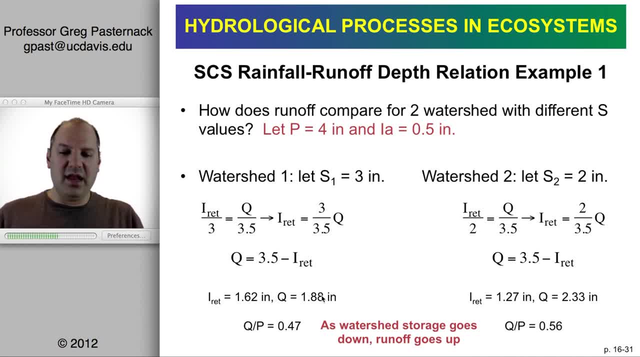 And what we find is the numbers that are given here and then, if we do Q over P, we can find out that the fraction of total water that you know the net, well, let's see. yeah, the fraction of the total water that rains down out of the sky, that actually runs off, is 0.47 or 47%. 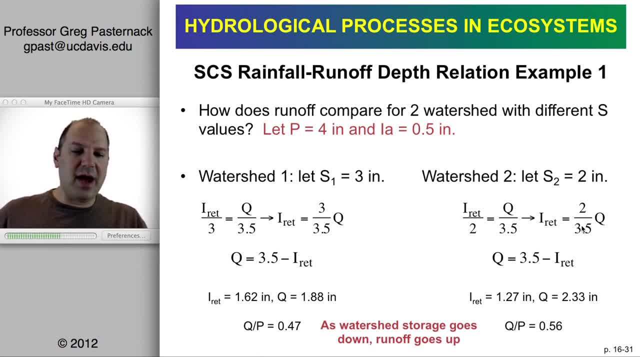 If we come to watershed two, we go through the same process. We just put in a two instead of a three and we find out that we get more runoff. So you know, the watershed has less soil storage capacity and as a result of that, you have less water retained in soil, more runoff and indeed a higher fraction of runoff. 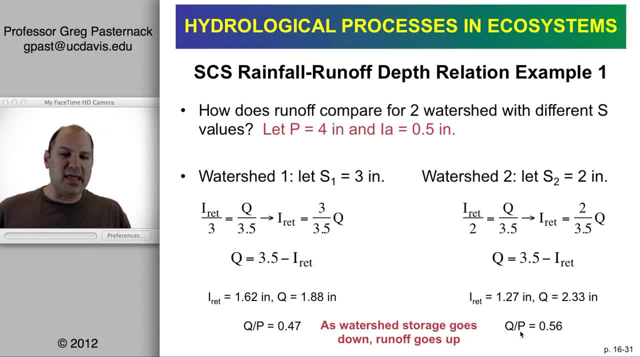 So I hope what you're beginning to see through this example is that the proportionality creates a very common sense outcome. That is that if a watershed has less total storage of water capacity, you're going to get more runoff, And that's what this linearity 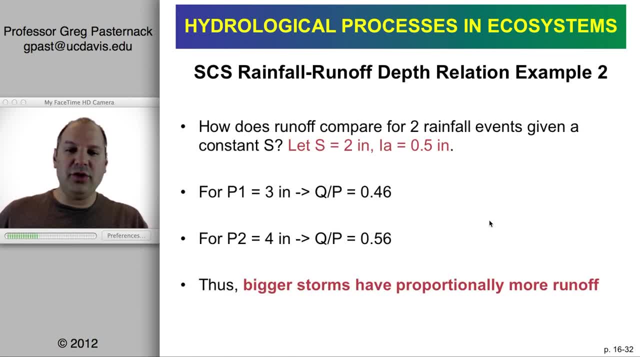 The other thing we could do is hold the storage constant and change the precipitation. So let S equal to the initial extraction remains 0.5, and then let's compare storms of three or four inches And you just put those numbers into the equations from before and solve, and you'll find that a small storm has a lower fraction of runoff and a large storm has a higher fraction of runoff. 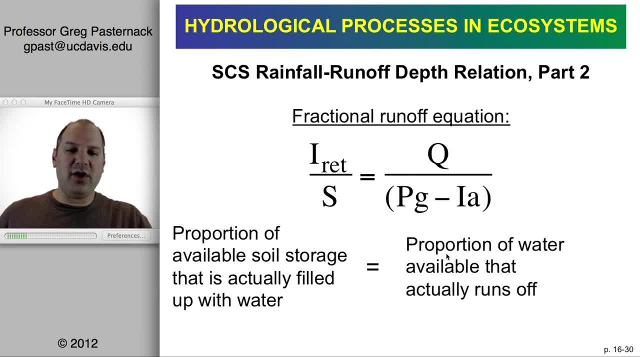 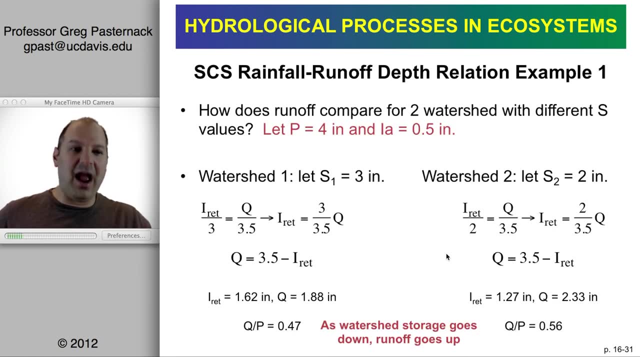 So, in essence, this very simple parallelism- It's just a matter of equations. you know, a mass flux equation and a simple rule, you know, for a linear runoff in proportion to linear storage- is getting at the key process for how watersheds actually might work. 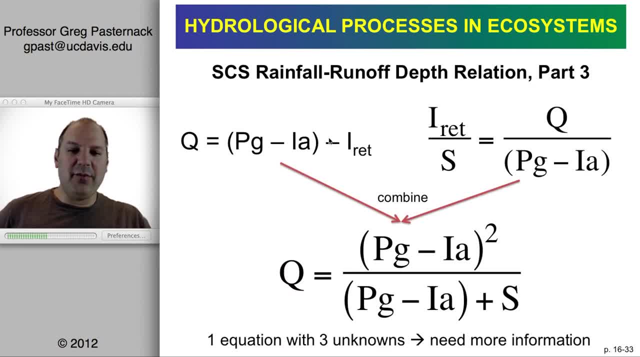 So if we take those two equations and we formally put them together, we can come up with this analytical solution that discharge equals a ratio of the net precipitation, PG minus IA squared. So if we take those two equations and we formally put them together, we can come up with this analytical solution that discharge equals a ratio of the net precipitation PG minus IA squared. 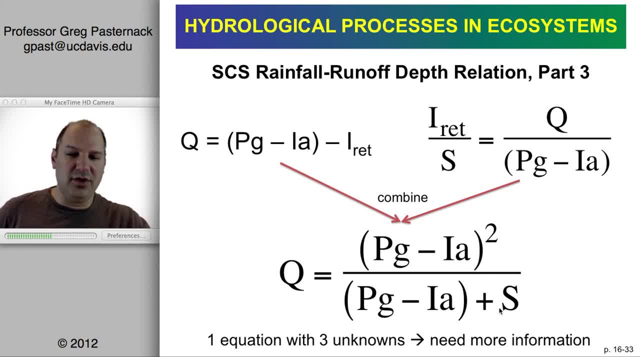 So if we take those two equations and we formally put them together, we can come up with this analytical solution: that discharge equals a ratio of the net precipitation, PG minus IA, squared divided by the net precipitation plus storage. and I'm not going to work through those steps. 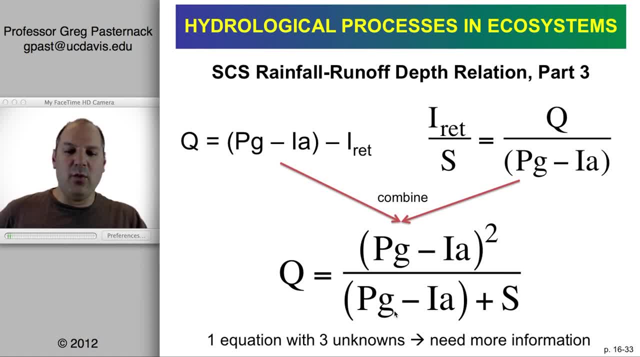 They're pretty easy algebraically. So the problem here is we have one equation with three unknowns: We don't know PG, we don't know IA and we don't know S. So this equation is not lumped enough. We have to do more lumping and more simplification. 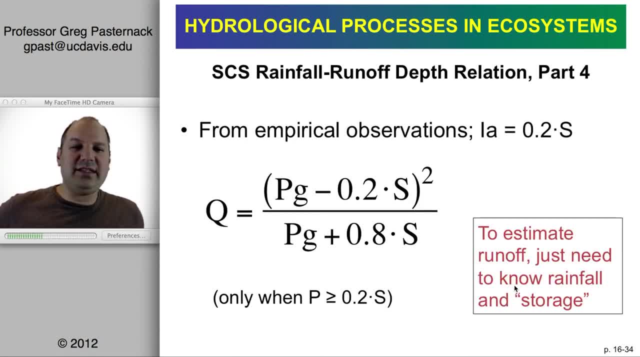 So the next thing is you send out all your scientists around the United States and you make measurements and you find out: hey, initial abstraction is actually related to storage and, in fact, initial abstraction equals 0.2 of the total storage capacity of the soils in the watershed. so, knowing that- and I 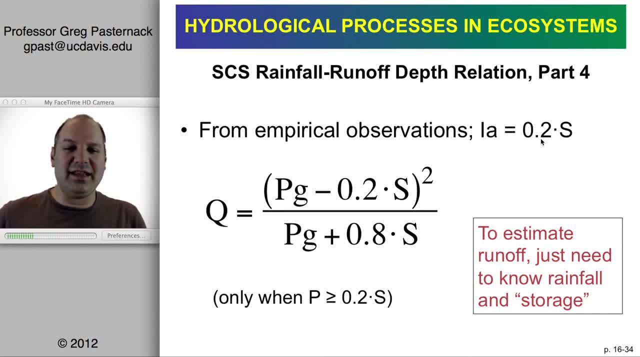 can only imagine what the scatter plot would look like for an analysis like that, but nevertheless, you can take that equation, substitute it in, and now we've reduced the equation down to two unknowns. so to estimate runoff. if we know what rainfall amount we're interested in, then all we have to do is: 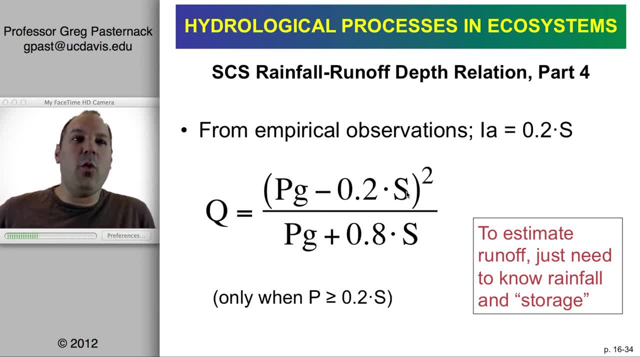 estimate something about s? how do you determine what that capacity is? and then you come to the realization that that storage isn't just a function of soil, but it's also a function of land cover and land use. now you may have highly permeable, highly porous soils, but if you have a- you know- parking lot over it, as 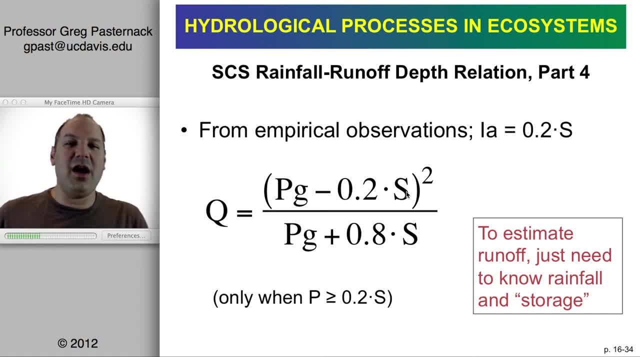 we've already covered in the class. you may have a highly permeable, highly porous soils, but if you have a- you know- parking lot over it, as we've already covered in the class- you're not going to get any run, any storage. so we have to have a way to. 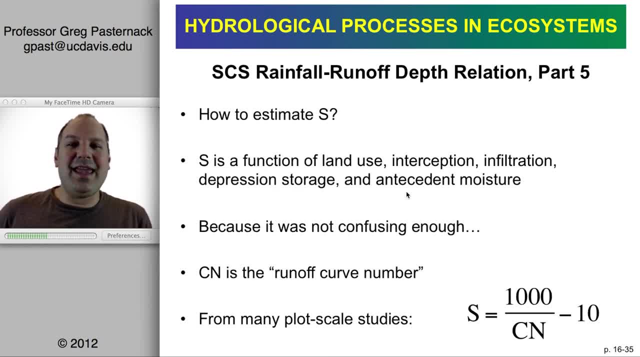 account for that. so now we're going to go again for another time to shift gears and try to characterize storage in terms of some land surface, land cover, soil characterization. to do that, the soil conservation service created the idea of a curve number, which is represented by these letters: CN. 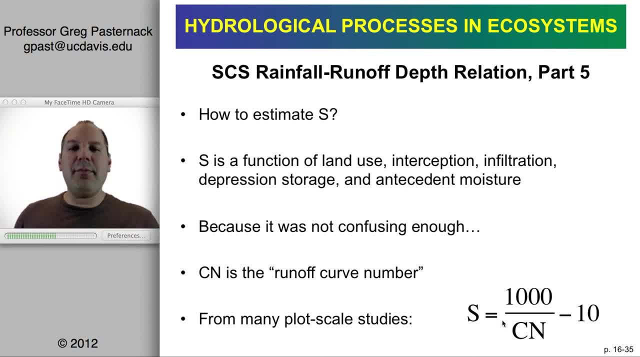 so curve number is something that you can look up in a table and I'm going to give you a handout that will show that, and it you find out that the soil storage equals 1000 C N minus 10. so this is an another empirical equation to get. 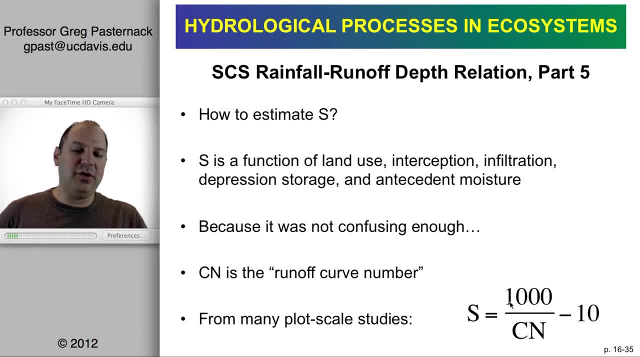 at, you know, a more tractable empirical, you know parameter that we can use to characterize the storage capacity of watersheds. so a curve number is something that you can look up in a table and I'm going to give you a handout that will show that. and you find, 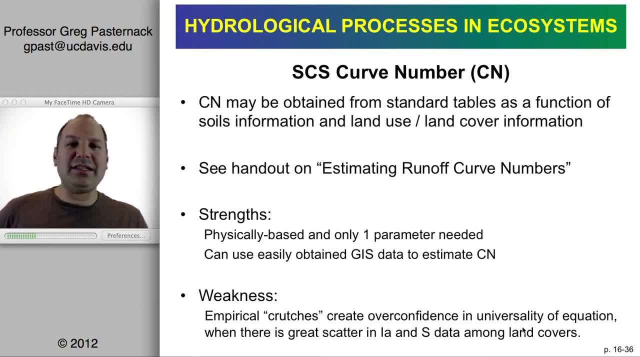 So what is this curve number? There are lots of standard tables. If you go into Google or you look up a hydrology textbook, you'll find these tables. It'll tell you that you know. if you're a residential neighborhood, you have a curve number of 70.. 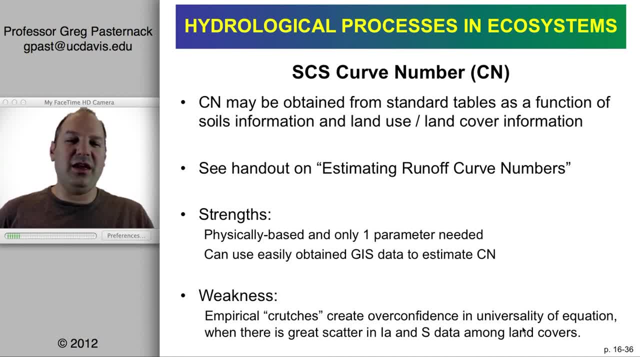 You know, if you have this soil type, you have a curve number of 40 and so on, And so I'm going to provide the class with a handout on estimating runoff curve numbers And you'll see that it's a function of land cover, land use and soil characteristics. 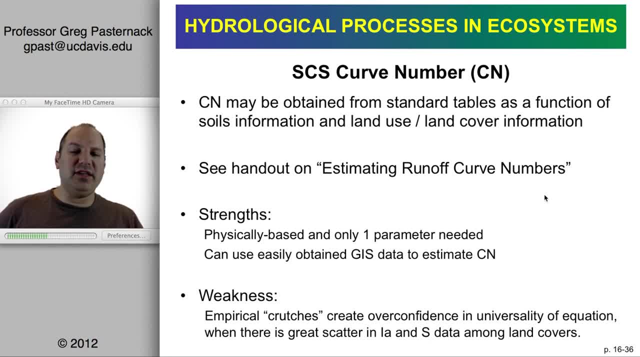 So, overall, you've got the whole arc of this thing. You've got two equations, one of which is a water balance equation, One of which is like a transport type rule, And you're putting that together with a whole lot of empiricism to make it tractable. 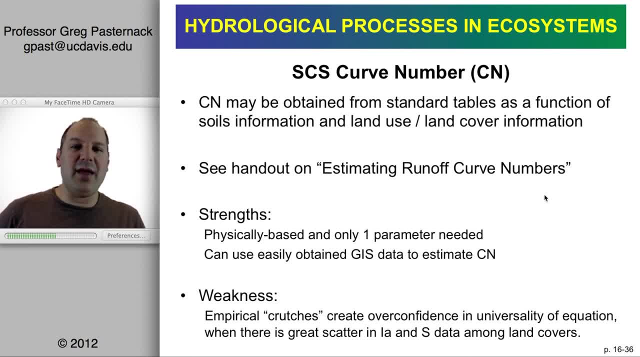 And in the end you have to just say something about the land cover type, again lumped for the whole watershed, and feed that in So it's not like, oh, part of the watershed is urban and part is rural, Like the whole patchwork thing that has been the basis of this whole class. 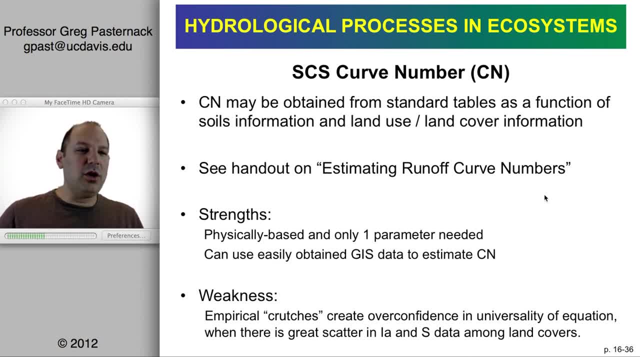 just throw that all out the window, for right now. You know you have to somehow aggregate all of that up and get one number, one curve number, to represent the watershed. So the nice thing about this is it does include some physical ideas. 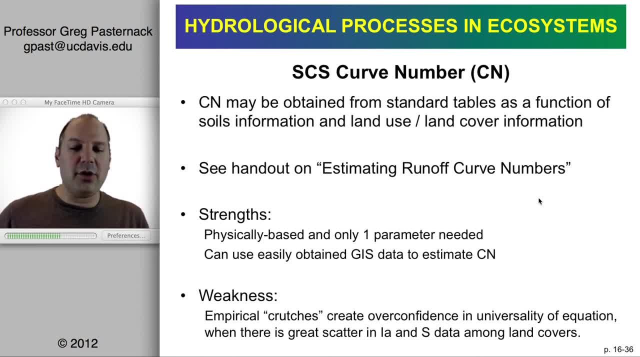 It is deterministic. It only has one parameter in the curve number, which is easily obtained in GIS, And you'll be going through an assignment not using GIS but to do that manually. The weakness is that it's got a whole lot of empirical crutches. 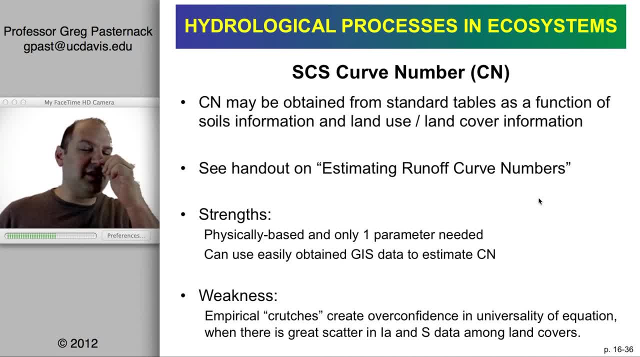 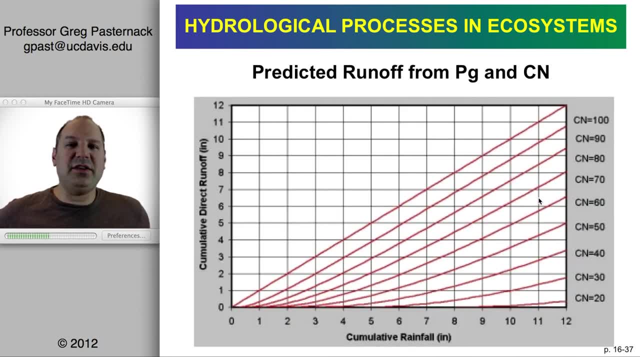 That are black boxes that most people have no idea what's in there, And then when you look in there, there's a lot of limitations that come into play. This is a graph that just conceptually illustrates the outcome of the curve number approach. 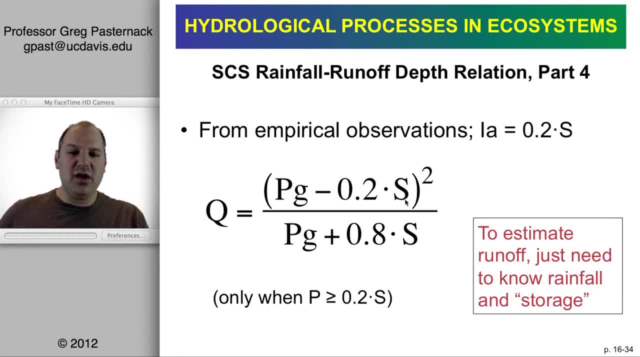 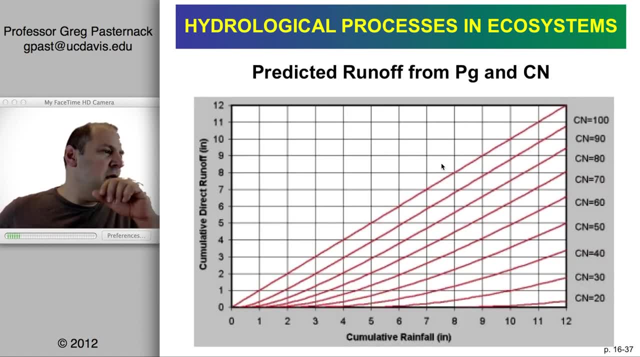 It's a non-linear outcome in the end because, of course, when you look here, you have this square And so it's going to have to be a non-linear result. But what you can see is that for any given rainfall, let's say you have six inches of rainfall and let's say you have a curve number of 60.. 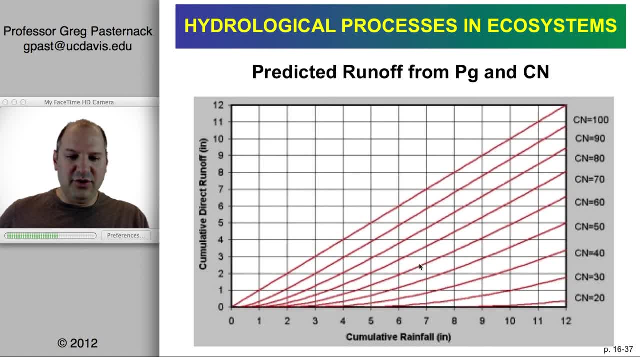 So I go along that curve number, come down to a rainfall of six and I find that my cumulative direct runoff is going to be two inches. So if I increase the rainfall from six to seven and I stay along that same curve number, 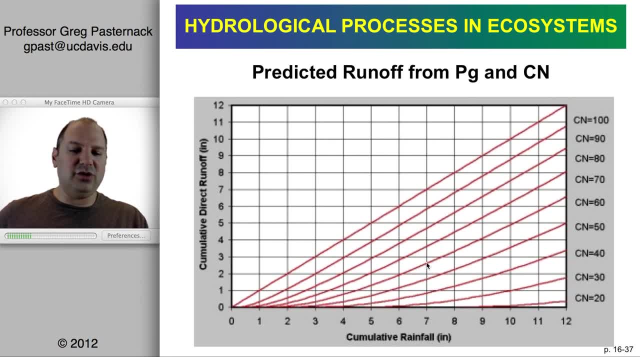 because I'm not changing the land, then you arrive at here, like you know, 2.7 or whatever. On the other hand, if I have six inches of rain, but then I urbanize and I go from, like you know that, two inches of runoff and I go to a curve number of 100,. 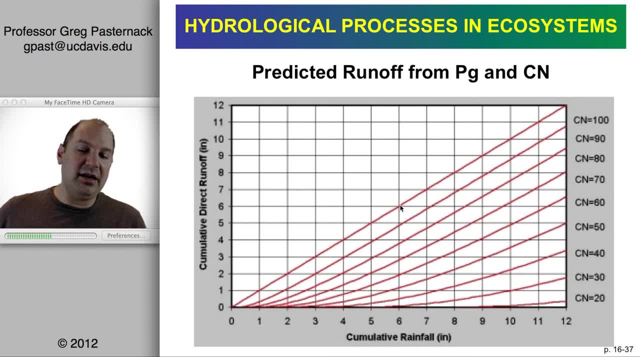 then I get six inches of runoff, which is three times, And actually that sounds pretty reasonable from some of the numbers that we've seen on the effects of urbanization. Okay, so what I'm going to do is I'm going to give you an opportunity for extra credit in the class. 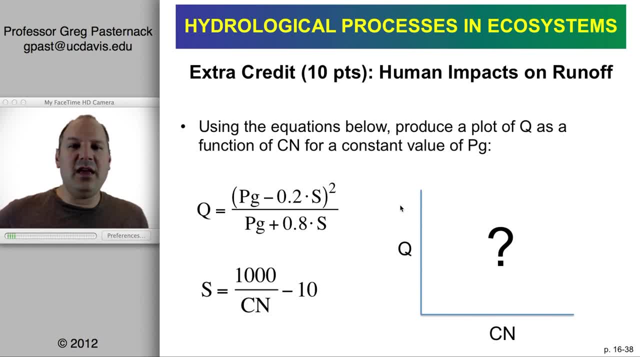 which is: take the equations that are shown on the slide and solve them to produce a graph with curve number on the x-axis, and then I'm going to give you an opportunity for extra credit in the class, which is: take the equations that are shown on the slide. 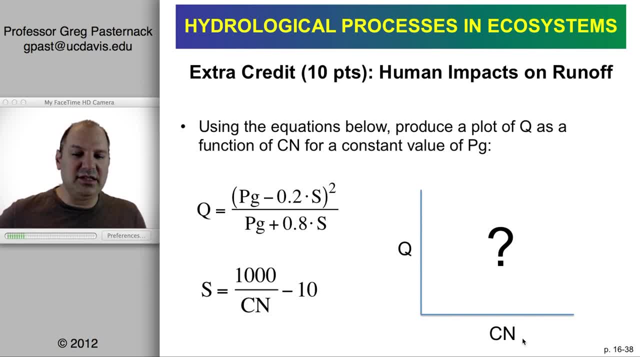 and solve them to produce a graph with curve number on the x-axis and discharge on the y-axis For the gross precipitation. why don't you pick a value of like seven inches of rainfall, let's say, and for a range of curve numbers, find out what is the runoff? 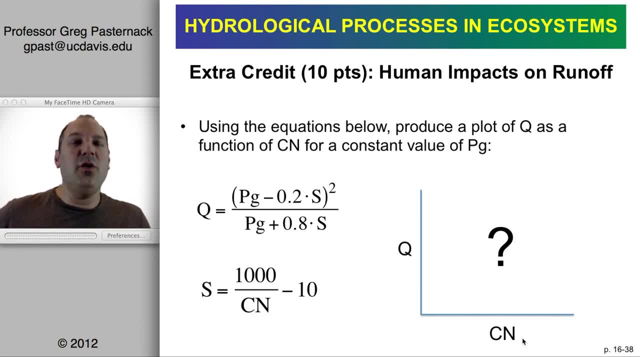 Now why am I asking you to do this as a bonus? The reason is that one of the themes of the class is to look at the effects of human activities on hydrological cycle and eco-hydrology. Well, the curve number is a bonus. 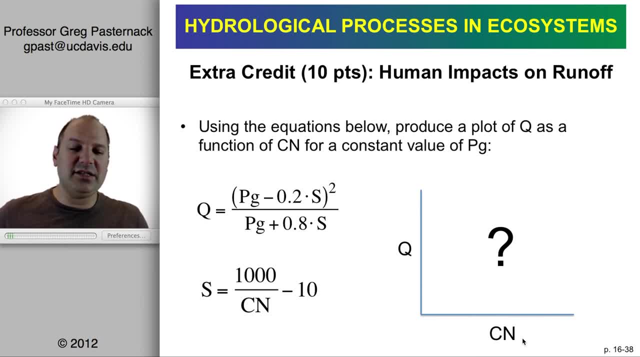 The curve number is this model's way of representing those impacts. So you can imagine a curve number for a natural- you know- well-forested landscape with patches of wetlands and everything else might have a low curve number of like 30, whereas like a- you know- agricultural grassland with a lot of- you know. 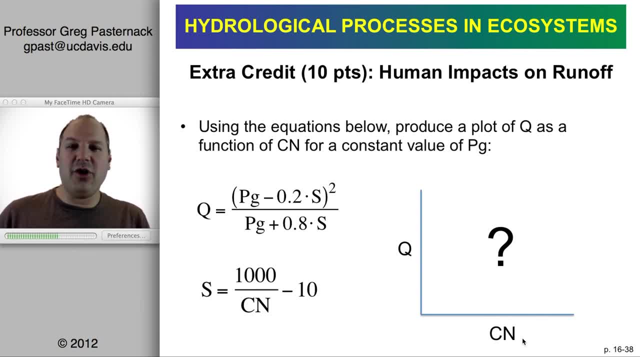 cows that have stamped down on the ground might have a curve number of 70 to 80, and then, you know, an urban area with a lot of pavement might have 90 to 100.. So one way to assess the effects of human impacts on runoff would be to see as curve number increases. 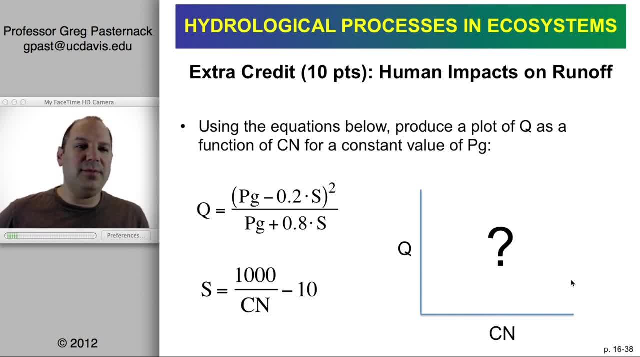 what's the change in discharge through time? So that's one way to look at it and you can pretty much recast all of the questions we've asked about urban into a format where you could answer it with: I'm sorry, not just urban, but deforestation, like all the human impacts. 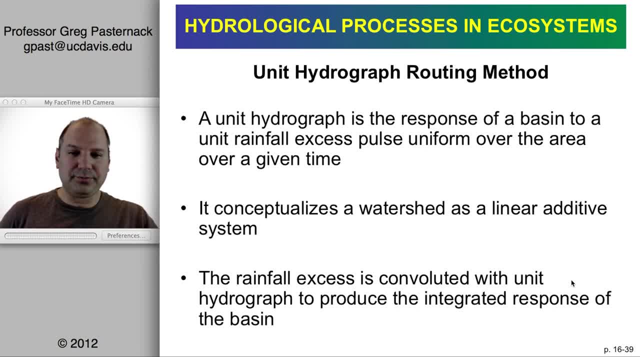 You could assess that in terms of this model. Okay, So everything I've been talking about there we've covered: how do you get the rainfall and then how do you go from rainfall to runoff. But now you've got the runoff at the mouth of that watershed. 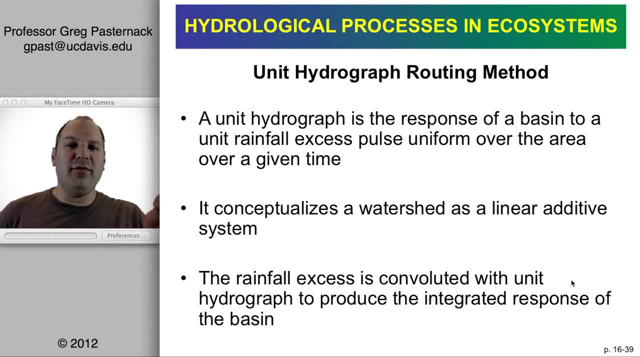 and now, potentially, you may need to move the water from the mouth of that watershed down through the river quarter to some other outlet. right, You could just have one overall lumped model for a whole watershed and just boom, you're done. Or you could break the watershed up into smaller sections. 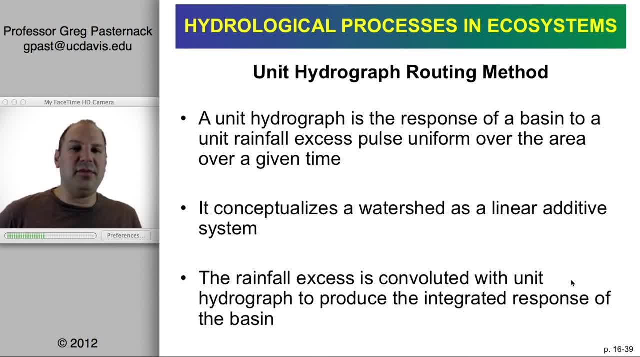 You could break it down into subbasins and then route the water from one basin down to the mouth of a larger basin, And that's a process called routing, And it would be beyond the scope of this class to go into the methods of how a unit hydrograph 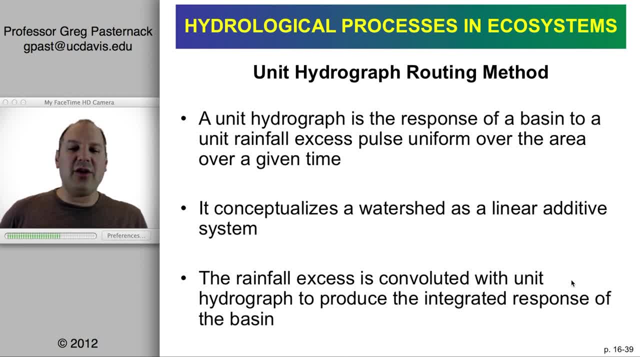 what is a unit hydrograph and how does it work? But a unit hydrograph, just to summarize here, it's the response of a basin to a unit of rainfall excess that's uniformly distributed over the area over a given time. I actually gave this definition in the urban lecture. 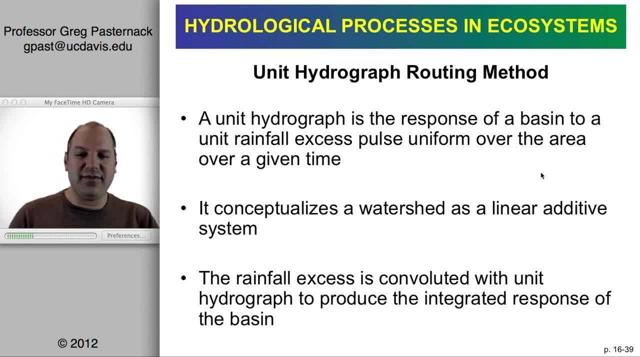 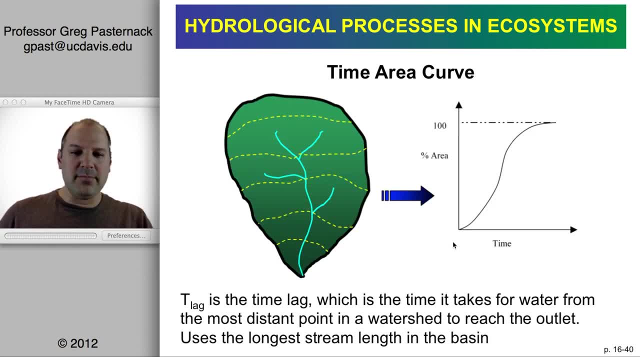 but it's. it's not a high priority and we're not going to go through the process of how this is all computed, But the important thing is it's treating the watershed as a linear additive system, So you can imagine there's there's a couple of ingredients that we need to figure out for this to work. 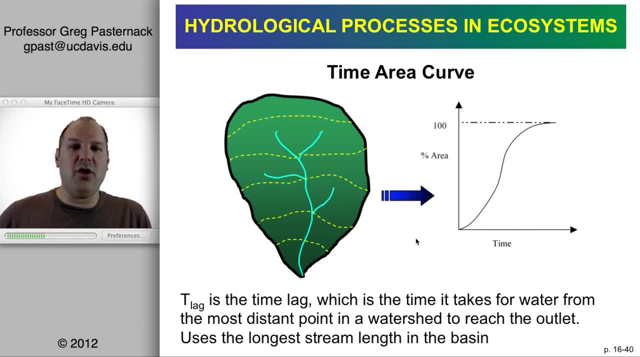 What's the peak of the runoff going to be for whatever we want to know. And then, when does that come? And so, to get to this time thing, you need some way to compute a variable known as the time lag. Time lag is the time. 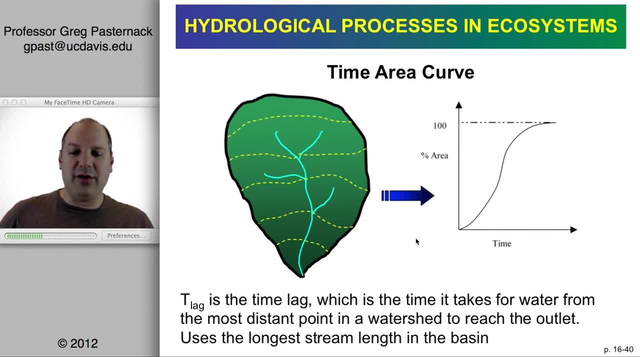 It takes for water from the most distant point in a watershed to reach the outlet. So that means, if you know, if I were to start like I don't know, maybe this is the most distant spot. Water is going to move relatively slowly to get to the stream head. 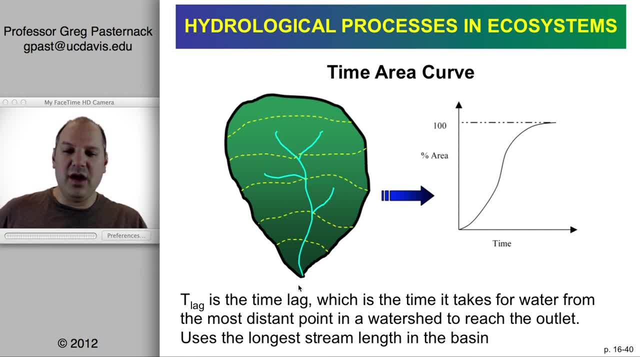 And then from there it might move relatively quickly to get to the mouth, Um, whereas somewhere over on the side it might take actually even longer because it's got to go over land quite a long ways and then it hits the stream. So it's not actually just. 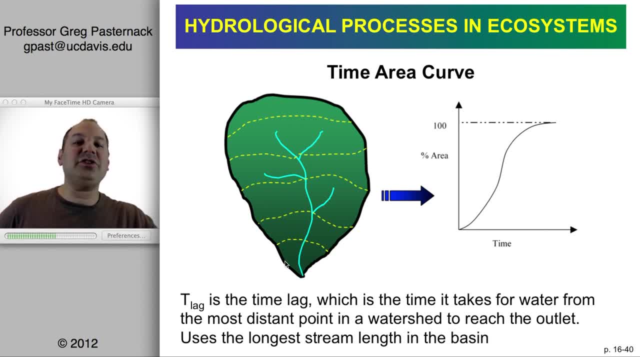 it's not the physically most distant point, but it's the hydrologically most distance point. And this is just a graph that shows, like um, the time, the, the amount of a watershed that, uh, it takes each interval of time to receive the water from. 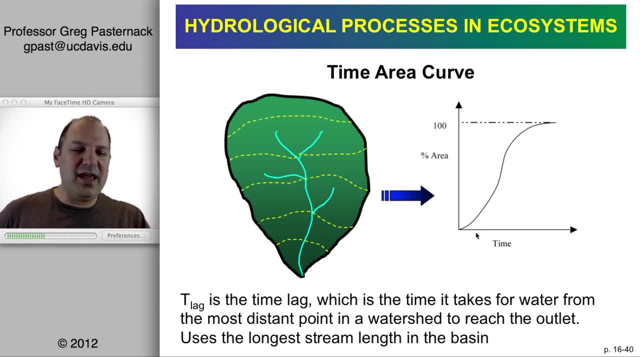 I, I didn't say that very well. Okay, let's try again. So, um, for each time, like, uh, let's say it takes one hour, like how much of the watershed can contribute its water in one hour. 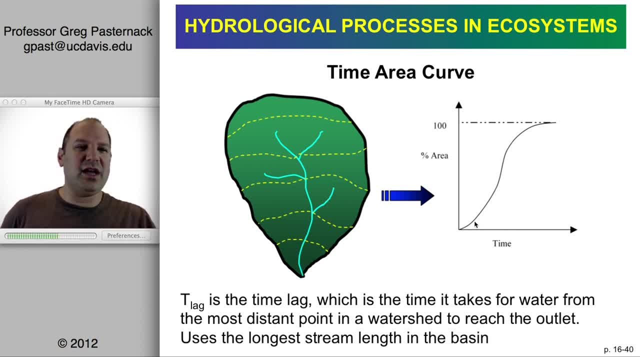 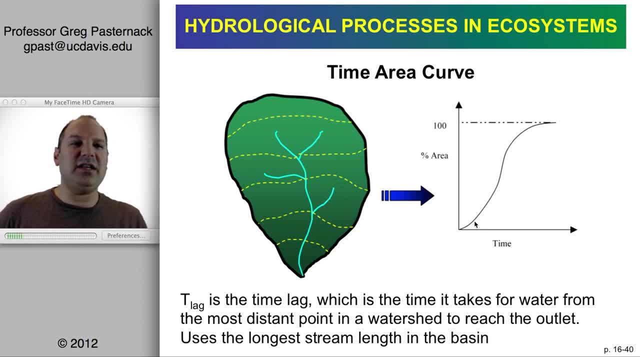 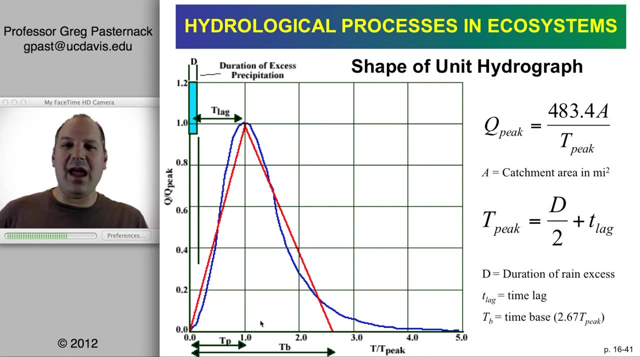 Okay, Okay, Okay. So this is a cumulative distribution function that gives us the percent area contributing water for each amount of time that you're interested in knowing. I think that's a better explanation. Okay, So here's a hydrograph. You're all familiar with hydrograph. on the X axis is time. on the Y axis is flow. 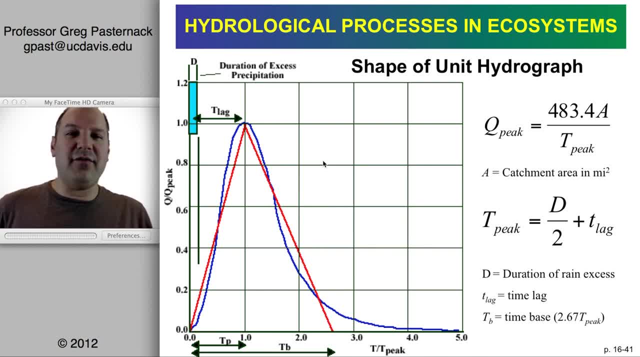 The blue curve shows a real hydrograph. Now for a hydrological model. does it really matter? the pure, exact, nonlinear shape of the hydrograph? If it does, this is the wrong model for you. but in most cases it doesn't really matter. 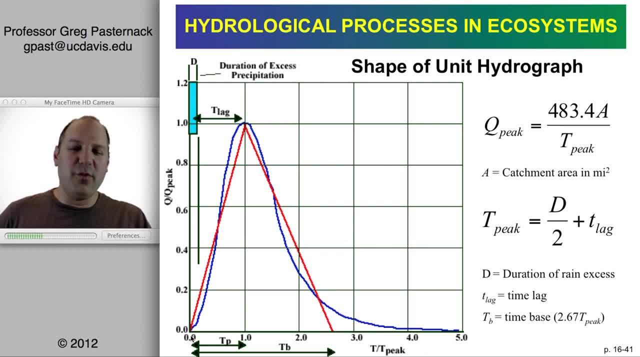 And so, with the kind of modeling I'm showing you, we represent the hydrograph as a triangle. Okay, And so with this triangle, the variables that matter are the time lag, which you know. it's shown here. The time lag is from the beginning of excess precipitation. 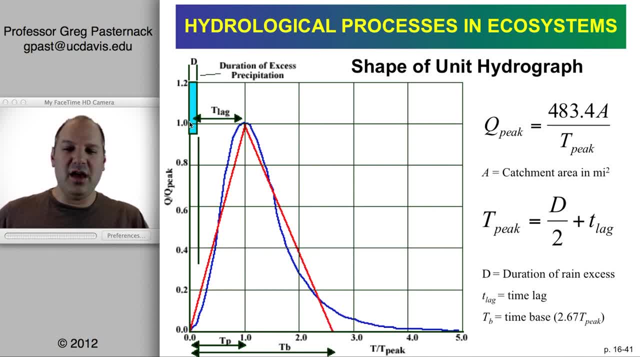 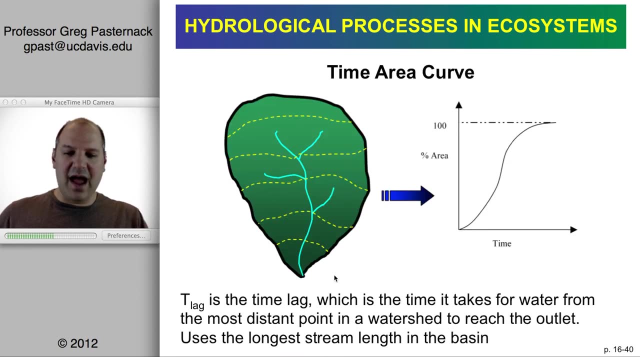 That's actually running off after initial abstractions are done until the peak, And then let's say: that's how the time lag is being represented here, And then we have the actual peak. So what is the peak? So here I talked about the time lag. 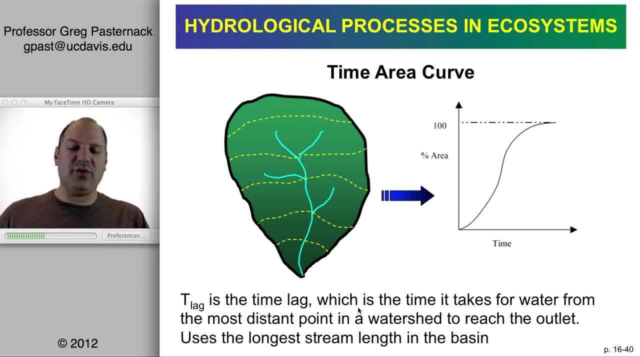 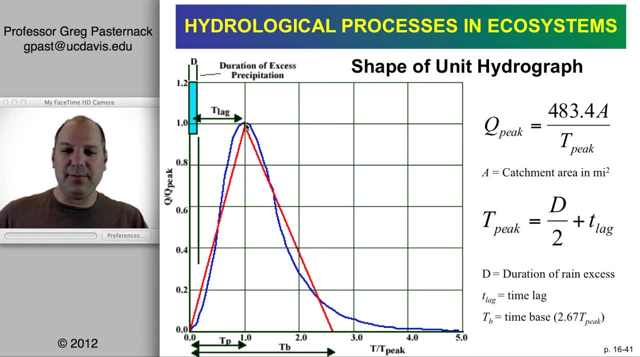 It's the time it takes for water from the most distance point to reach the outlet. Presumably, when that's happening, it's going to be associated with the peak, but maybe it's not always that way. So the way, oh ah. 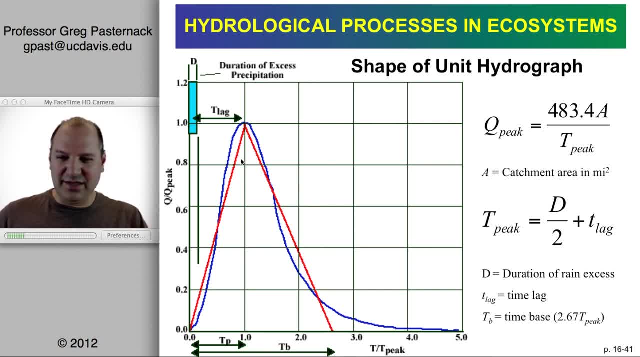 okay, now I got it. Time to peak, There we go, Okay, So. so time to peak is the time. That's where we're at. the time to peak is the time that's going from the onset of rainfall excess until the peak. 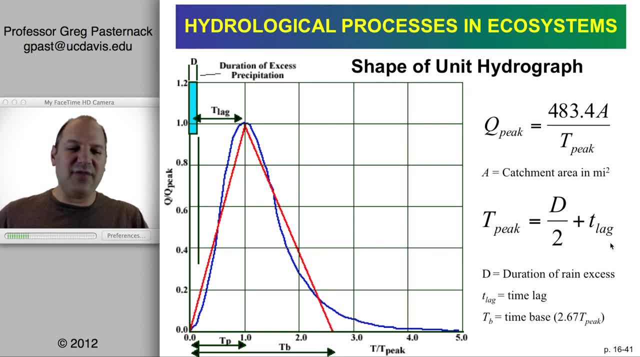 right. So that's time to peak, And it is- it's a function of the time lag as well. Okay, So so there are some empirical equations that are used here to get at this again, based on studies that have been done. 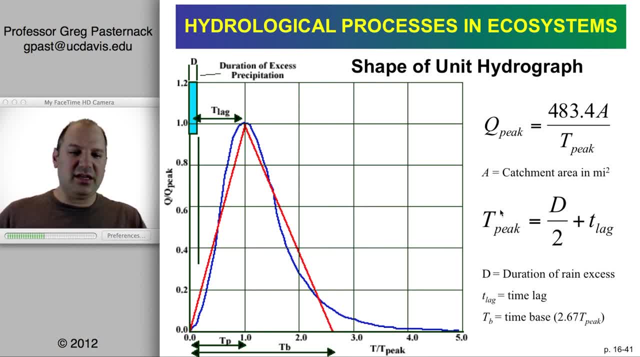 So you start by calculating to time to peak as the duration of rainfall excess precipitation divided by time to peak, Okay, Divided by two plus the time lag. And then you take that time to peak, you put it into this function here and you get the peak discharge equals 483.4 times a over T peak. 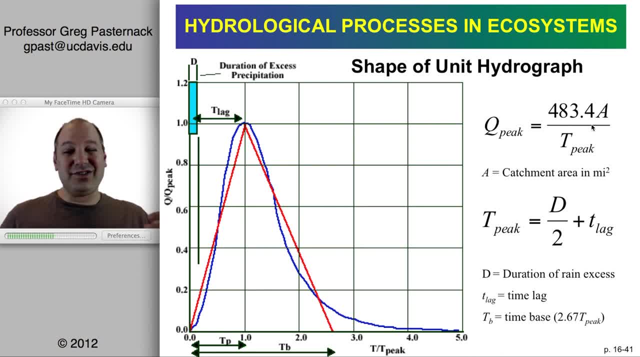 So there's a lot more detail that you could go into to try to understand why it is the way this is. to do that, I'll be showing you some manuals that we'll be going into that more And that's just beyond the scope of the class. 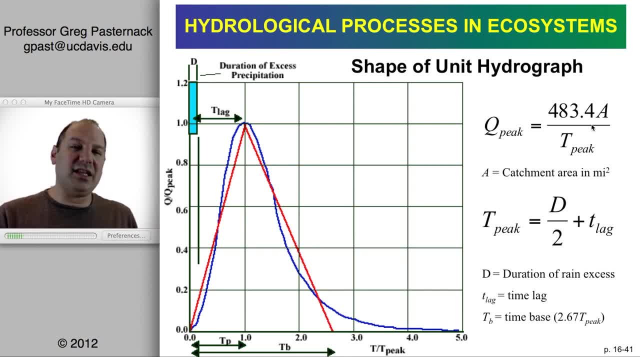 because what I really want you to do with this model is to just get the conceptual idea of it, that we can represent the hydrograph in terms of a peak discharge and a time to peak, And then we can take that and use that to run the model. 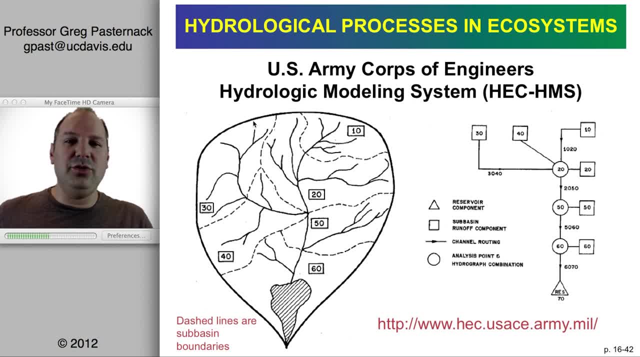 And the model that we're going to be playing with is a very standard model used in consulting and professional hydrologic project practice in the United States, which is the United States Army Corps of Engineers hydrological modeling system. So there's a branch of the army. 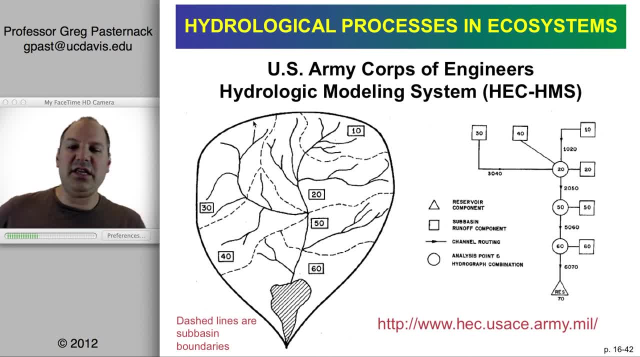 That's called the hydrologic Hydraulic engineering center, HEC. It's actually located here in Davis, California, And the HEC has a model that today is called HMS. Historically it was called heck one, and heck one is the most simple. 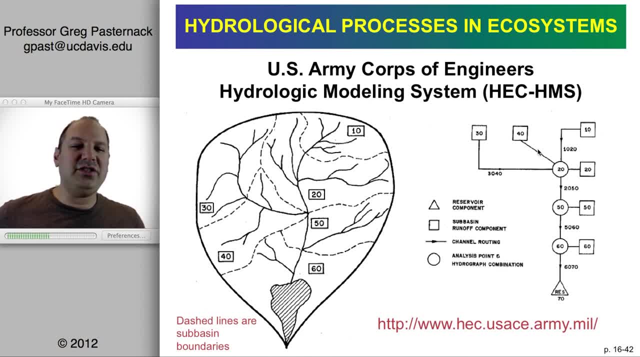 you know efficient way to go. Heck HMS has a nice user interface and you know a little bit more graphical button pushing, but the nuts and bolts are still essentially what's in heck. one is just added a lot more bells and whistles and 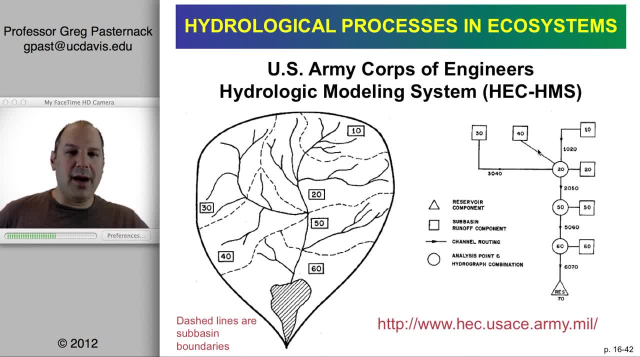 and ways Of looking at it. So what you do with a lumped model like heck HMS is you take your watershed, as shown here in the schematic, and then we're going to divide that into sub basins. Now the hard part that you really need to understand is that the sub base and delineation the 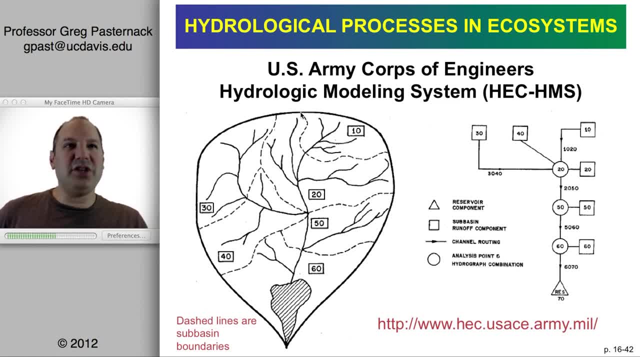 that these basins can be. let's say, each basin has a unique area, but water from one sub base and can flow into another. So, for example, let's look at this sub base in 10.. Okay, Here the dash line represents the watershed boundary for that. 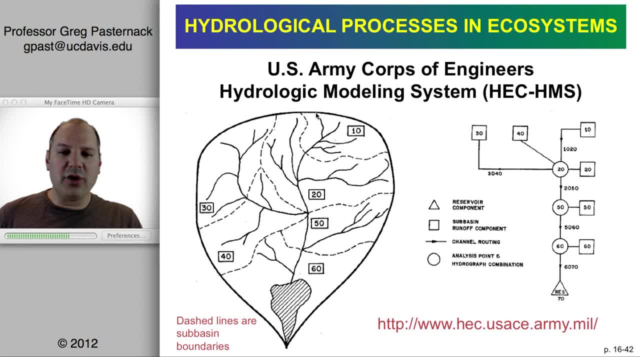 So water cannot flow across the dash line. All water within area 10 is going to come to this one outlet point at the channel. from there The water is going to have to be routed to the next point, which is the mouth of 20.. 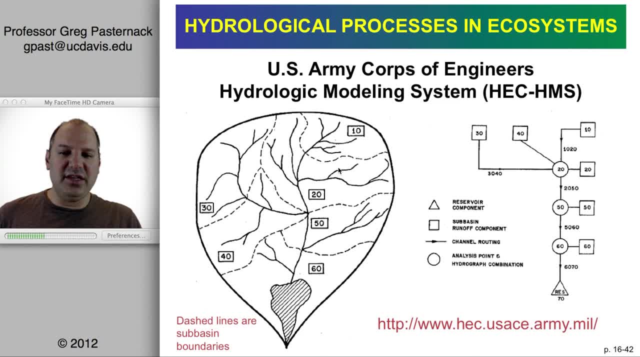 So 20 is this, is this strip that's bounded by these two dash lines, And you know that area. then you compute the amount of water contributed there, And so you can. you can see each one of these has its own area. 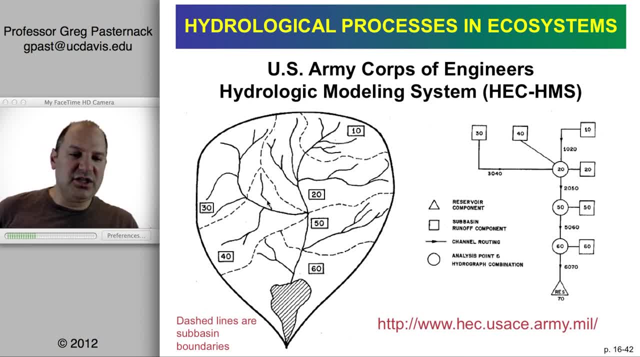 And then how flow moves from one to another is represented in the schematic on the right. This is relatively similar to the kind of schematic I was asking you to draw for this- the Salinas river assignment- back when we were looking at range lands. I gave you that assignment to start preparing you to think about what you're looking at right now. 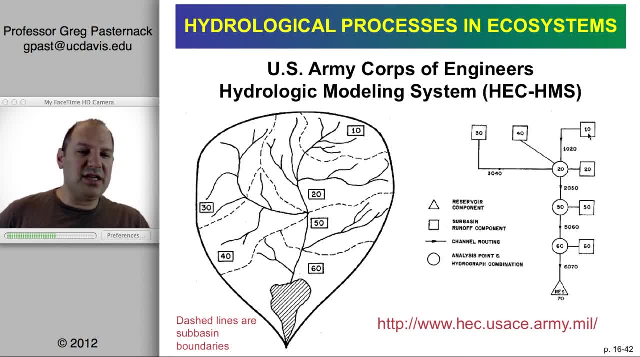 That was kind of foreshadowing this. So what you see here is like watershed: 10 flows into 20, 20 also receives water from 40 and 30. But in addition to that it generates its own water. So the squares here represent a rainfall runoff process. 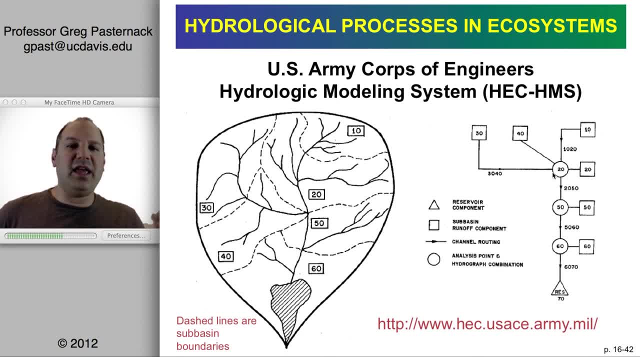 And then 20 represents a combination point where you're linearly adding all the water at each time step as it arrives at that point. Then water from 20 is routed down to 50.. 50 has its own water that it contributes. It routes all that to 60.. 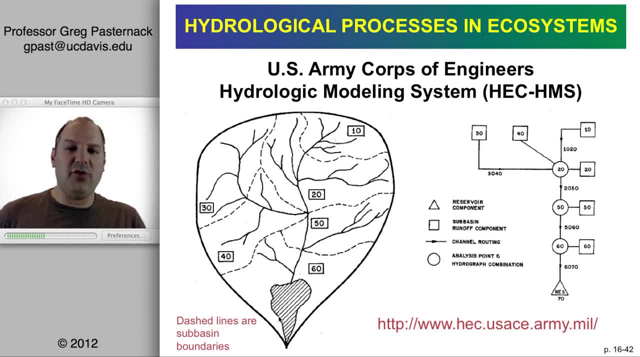 And then 60, adds its water and then down to the reservoir which is shown with the hatch line. So that's the general concept of how this model works. Again, until you're hands on with this, I know it's going to be hard to think about it. 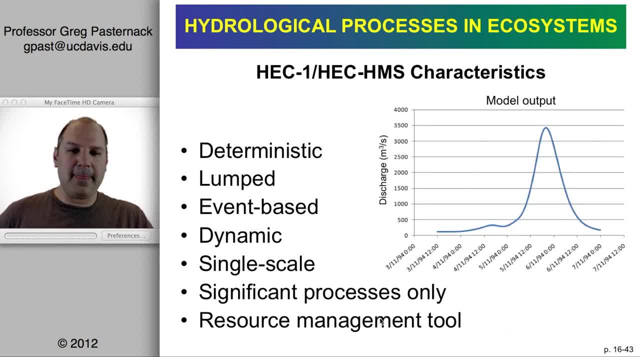 So we will, of course, have assignments that deal with this. This is what an output would look like from this type of model. You have discharge through time. It's a transient flow, It produces a hydrograph. So it's deterministic model as opposed to stochastic. 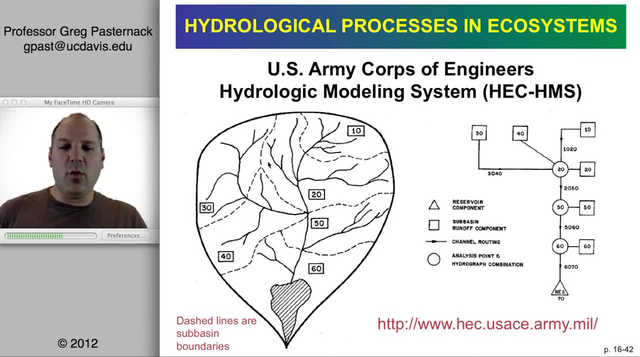 It's lumped in the sense that, you know, even though we break the watershed into a few sub basins, we're still treating large areas with one set of land cover numbers. So it's you know, it's spatially lumped and also process lumped. 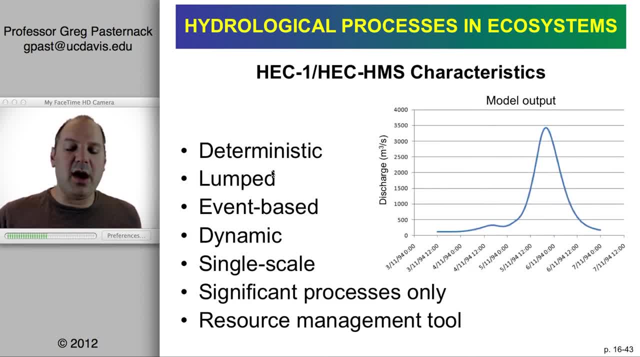 So there's two different ways of defining that concept of a lumped model. These models are generally event based because they don't track soil moisture through time. So you usually are going to use this to get one hydrograph dynamic And that it means it changes through time. 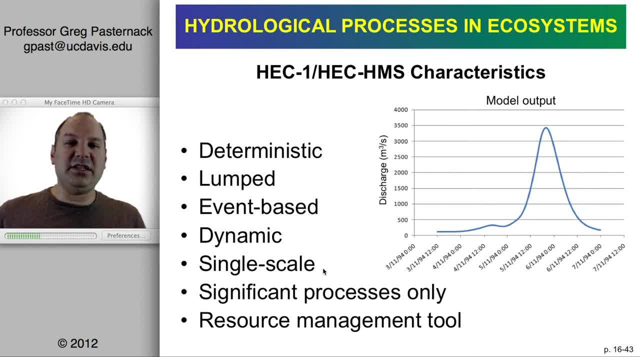 There's a single scale, which means that you know the processes of initial abstraction and you know soil storage and land cover effects. they're all rep. regardless of how big or small you make your watershed, you use the exact same equation. 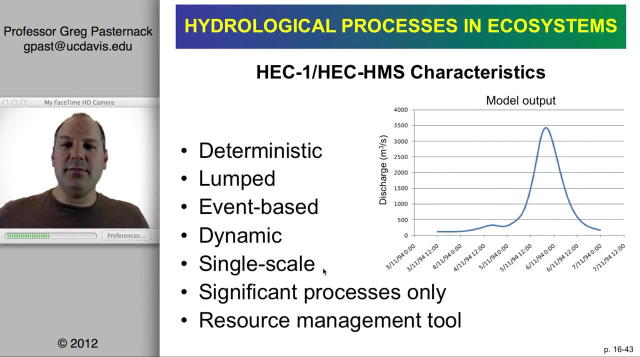 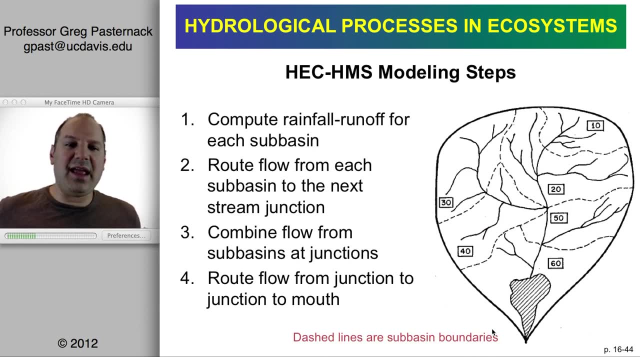 It's not scale dependent, It's only looking at the most significant processes. You know we've greatly simplified the physics of the problem and this is used as a resource management tool, not as a scientific exploration tool. So what are the steps in a HEC HMS model? 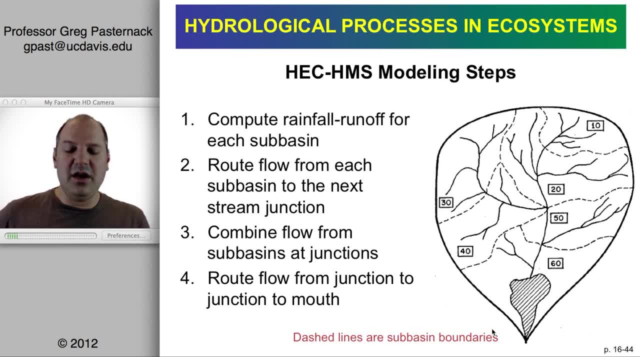 And of course you'll be doing these steps very soon. Compute the rainfall runoff for each sub basin, route flow from each sub basin to the next stream junction. combine flows from sub basins that are at that junction and the route flow from junction to junction down to the mouth. 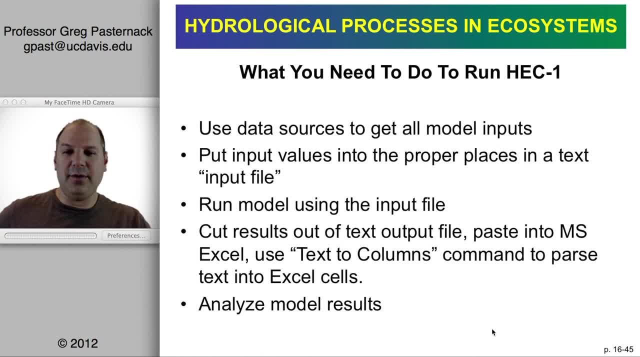 So I've already walked you through that once, but I'm just hitting it again In a nuts and bolts way. what do you need to do to actually run HEC, HMS or HEC one- And I'm kind of using those somewhat interchangeably- 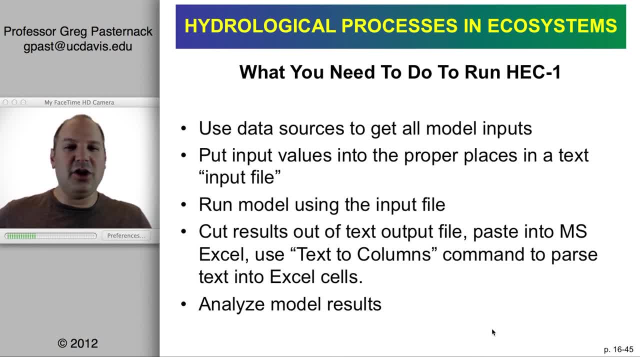 I mean, the more you go towards the graphical user interface, then the cookbook sort of changes. From my perspective it's really helpful to start with the most basic fundamental model in HEC one and understand how that works and then pick up the graphical elements on your own or in your job. 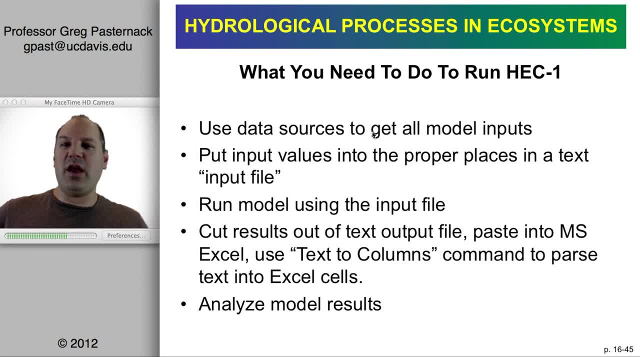 Of course you're going to need to take, get all your data sources. you know whatever information is going to drive the curve number care, your characterization and your precipitation information. What are the size of events that you're interested in? the hundred year event? 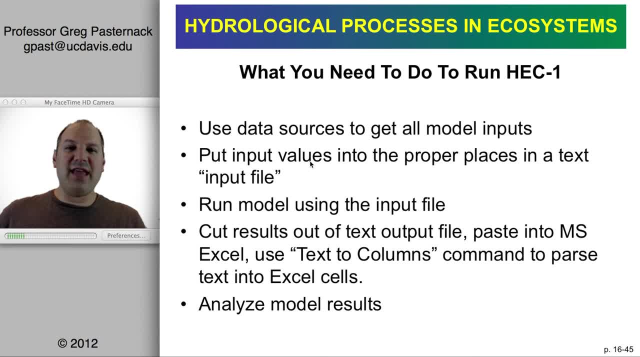 the 10 year event and so forth. Then we're going to have a text file. You're going to love this. You take all this information, you put it into a simple text file. If you're on a PC, that's going to be like notepad. 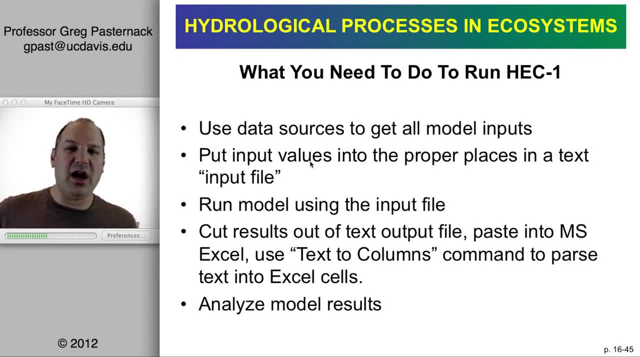 If you're on a Mac you can use text edit, but you can't run this software on a Mac, so you'll have to convert it over to a PC. You run the model. To run the model, so to speak, is not nothing magic about it. 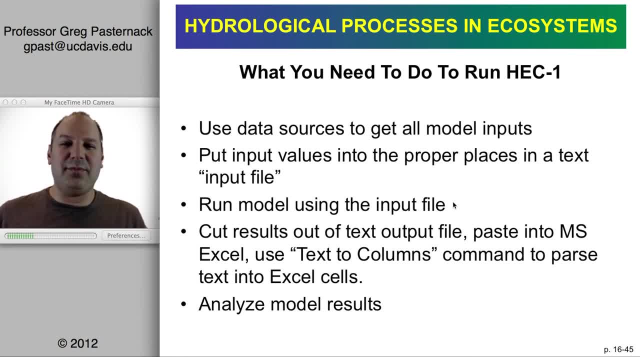 You just double click on an exe file on a PC. It reads the information from the input, It runs and produces the output. The output is another text file. You can copy and paste information out of that into Excel and, you know, parse the data out using a function in Excel called text to columns. 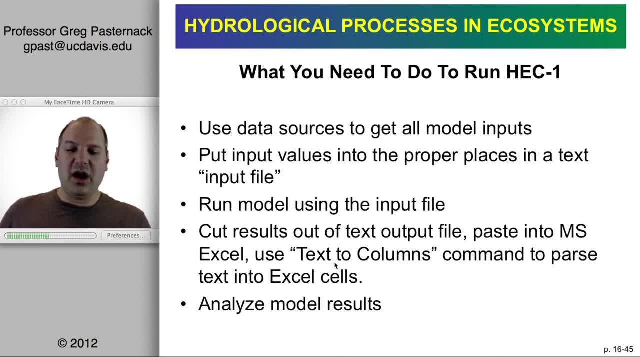 So don't manually type the numbers in. Of course, uh, with the graphical interface and heck HMS, you can produce a variety of outputs that can be directly used to generate graphs internally in that software or to bring it into other software. Um, 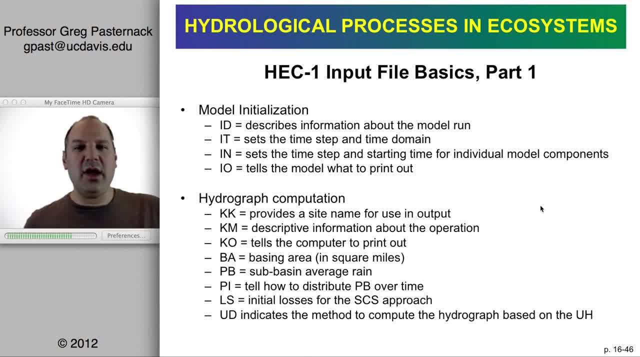 analyze model results. Okay, so imagine you know if you've never done any computer programming before. a computer program is nothing more than a line by line set of instructions telling a program what to do. Welcome to computer modeling. Um, the way heck one works is that each line in this text file begins with a two letter code that tells the model what to do. 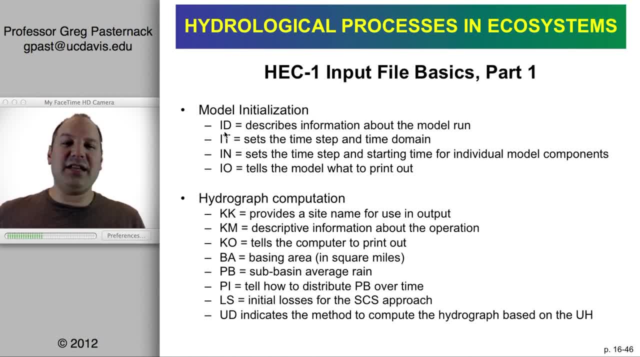 Um, the first code, like ID. it doesn't tell it anything, Just saying, Hey, here's the identification for that model run. it set the time step and in a few others. But the next part is we have to start computing the hydrographs and each one of these codes. 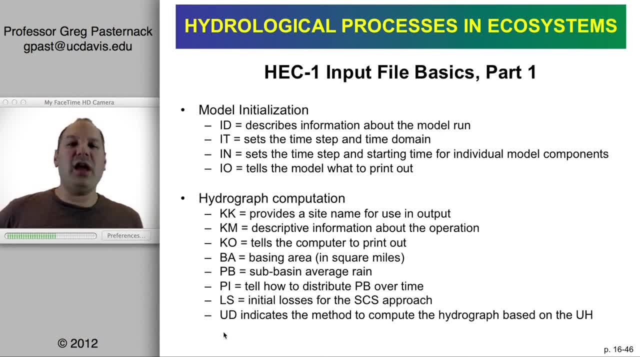 and I'm not going to read through them all, Um, but we'll work, be working on this, And, but we'll work, be working on this, And, but we'll work, be working on this. And you can look through both the heck one manual that I've provided for you, as well as these slides, to see the different kinds of things that you can do. 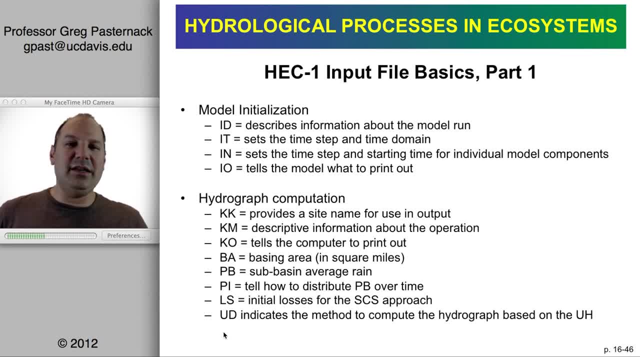 I'm going to provide you with a template file that has the basic nuts and bolts and placeholders, And then you just have to put the correct numbers for the sample data in to the files and run it. So there are codes where you're for each individual line. 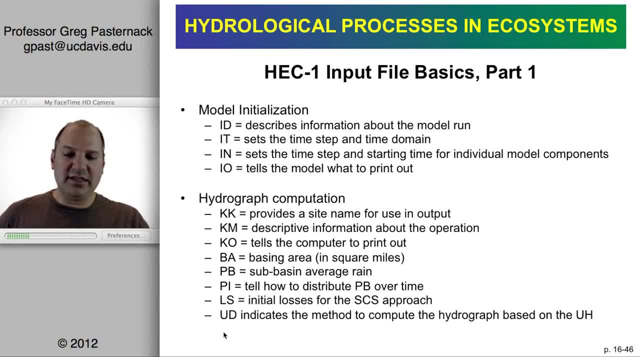 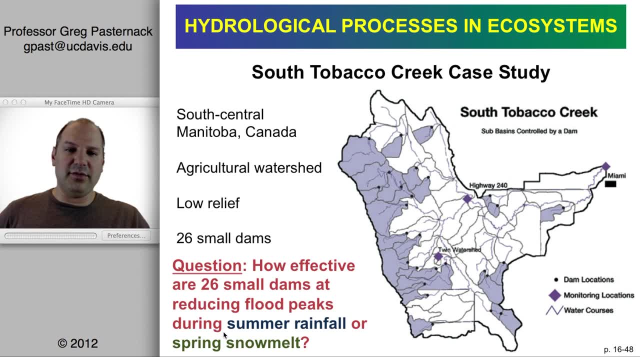 you're going to be computing the rainfall to runoff process. Then there there's going to be the hydrograph routing, mooting water down the system and then combining the hydrographs together. Let me just illustrate this with a practical example of what you might do in a consulting project. 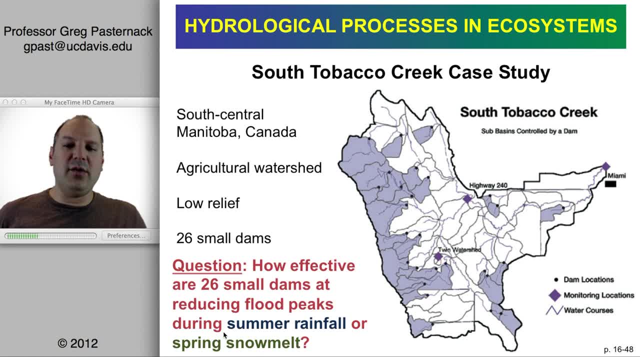 Here's an example that I found for South Tobacco Creek, which is located in South Central Manitoba, Canada. It's an agricultural watershed, low relief. Um, there's a lot of dams. If you look at this area, the outlet is where the diamond is. 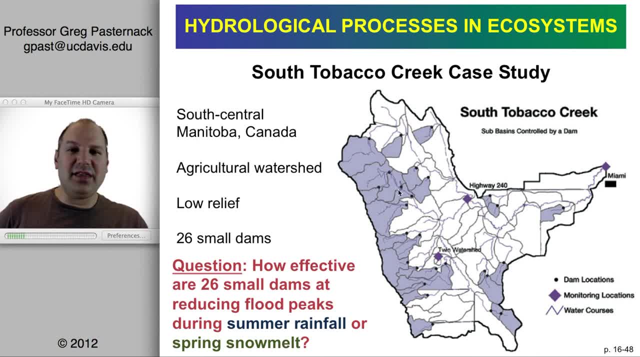 And then the black line is the watershed. Every black dot that you see is a dam in the system. And then, um, I I believe that the shaded kind of bluish area is the total area of land that is contributing. uh, 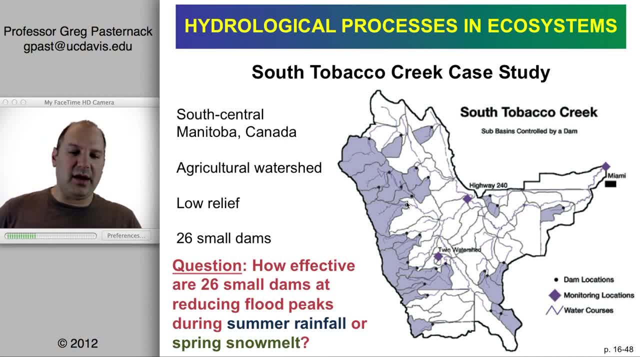 to a dam And then where it's white, those are areas that are unregulated. So the? so, given these 23, 26 small dams, you could ask a management question like: how effective at the are these dams at abating the instantaneous peaks associated with different return interval events? 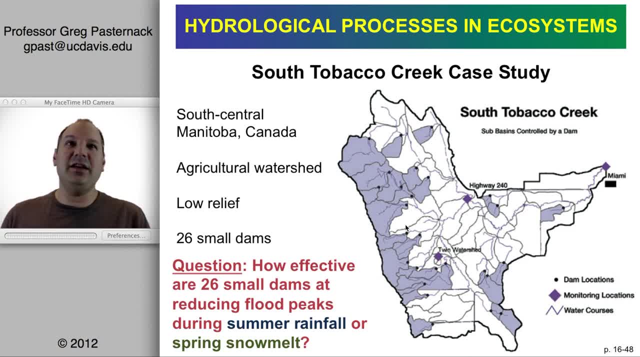 right Because, remember, the peaks are are going to hinge on the size of the event, and dams are just a form of storage. So you know very well by now that the hydrological effectiveness of storage is dependent on the frequency of the event. 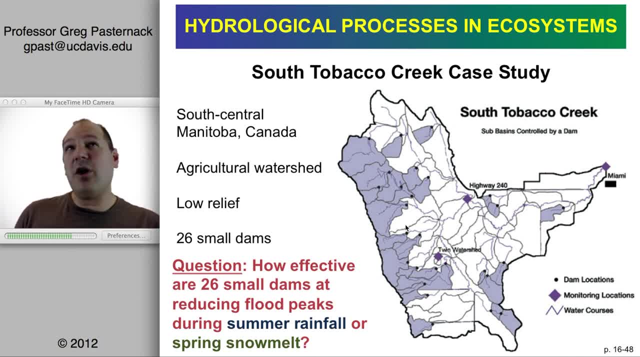 We could also ask the question: what if we were to switch from 26 small dams to one big dam? You know, maybe if we had one big dam we wouldn't be creating watershed effects all over the place. We could consolidate um. 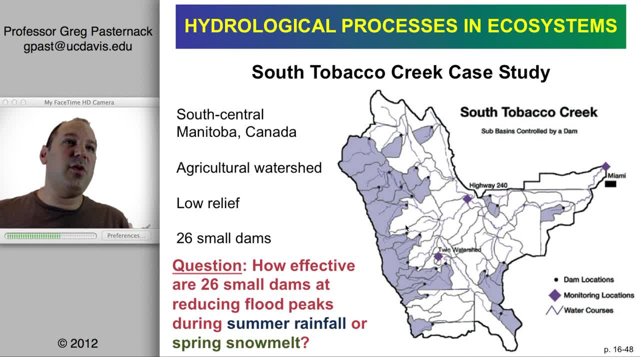 the damage, so to speak, into one area. Alternately, maybe 26 dams give us more flexibility to turn things on and off, whereas one dam can't be flexible at all. And then, finally, we're going to look at the effects for summer rainfall and spring snow melt. 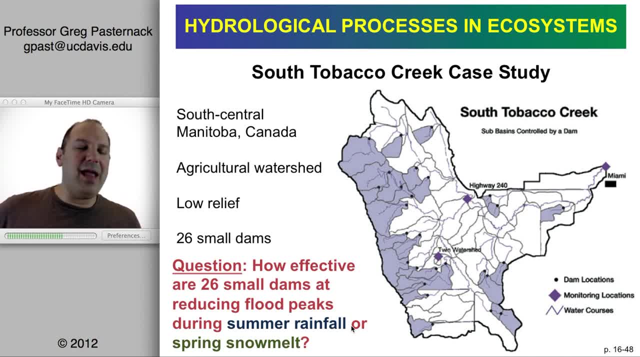 And I think what this example is going to show you, without a particular validation, but it's going to show you, in more of an exploratory mode, how a model is very useful at giving you an idea of of you know actual numbers for what the benefits are, or lack of benefits are. 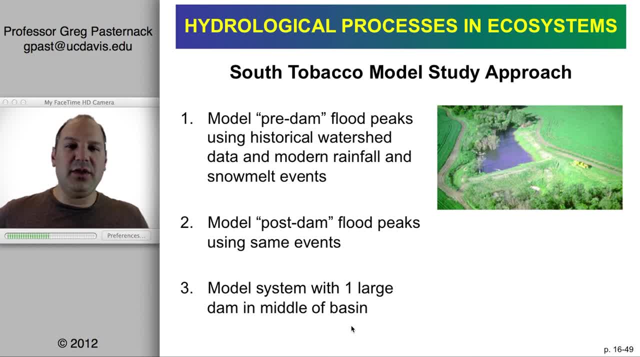 So we're going to model the pre-dam flood peaks with HEC-, HEC-HMS, using historical watershed data. Um, then we're going to model the post-dam peaks and um see what the differences are. The first step is we have the sub-basin area. 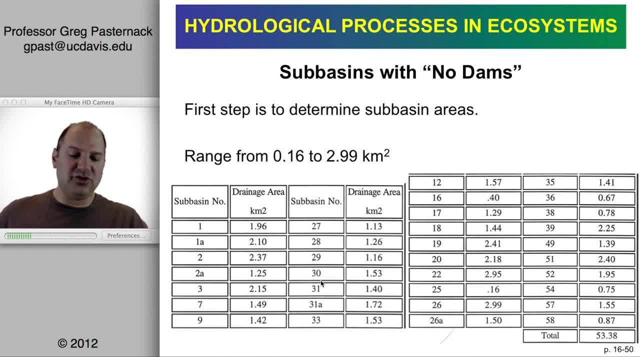 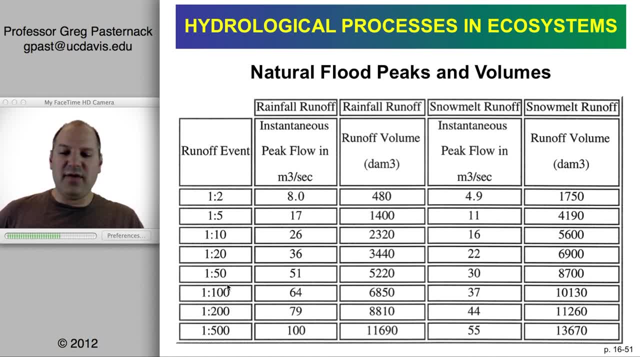 So here's the number of sub-basins and their contributing areas. Then we look for different runoff events. you know the uh, the one and two year event to one in 500 year event. What is the? the instantaneous peak flow. 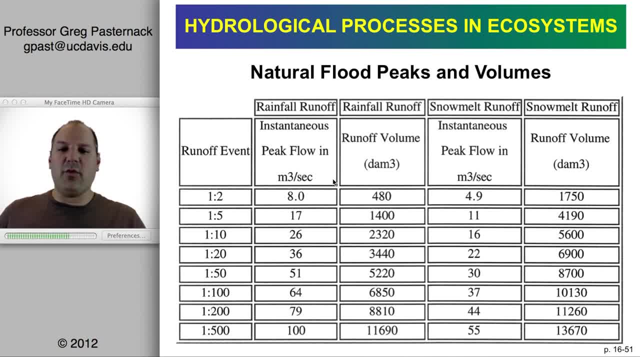 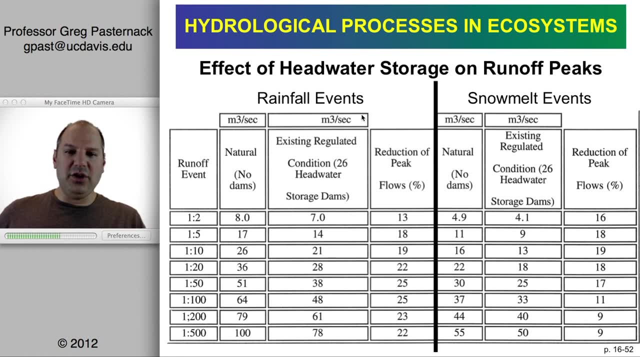 um, that results from the model in a rainfall runoff scenario, And then what's the total volume of want runoff? That's, that's there as well. Uh, and then we can do the same thing with the snow melt case. Okay, So the next thing we can do is we can put in our 26 dams. 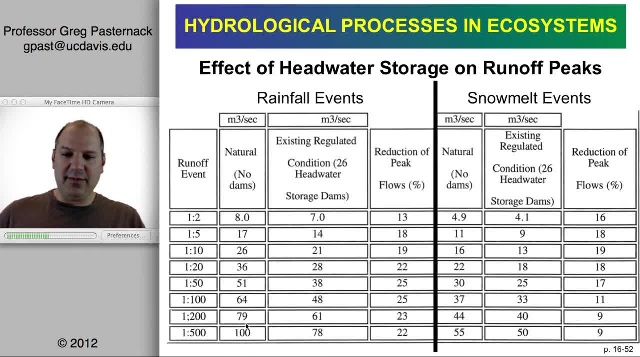 So we have the natural runoff that was there, And so that's the same. You see, this first column here is the exact same as the first column We had before. we can then put in the effect the results that come of including the dams. 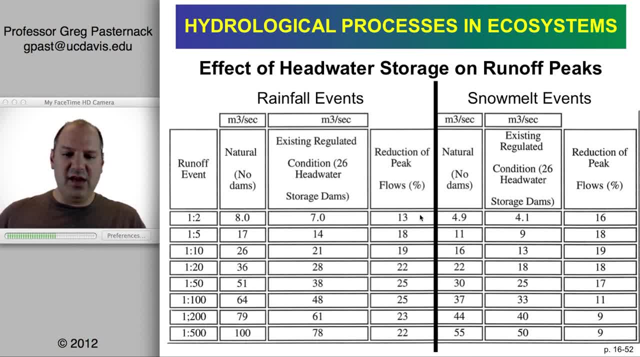 And the third column shows the reduction in peak flow. So you can see anywhere from 13% to 25% uh benefit in terms of percent reduced flows. Notice that, um, the the greatest benefit isn't necessarily associated with the smallest storms. 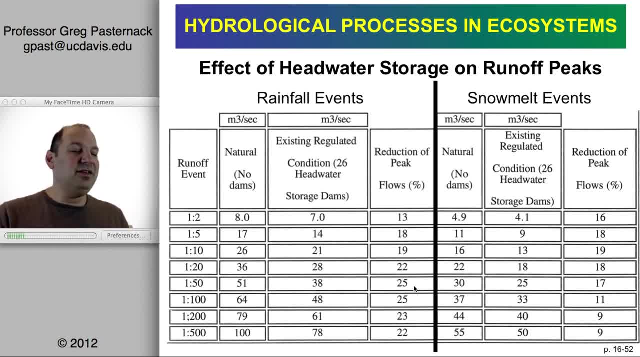 which is what I would have expected theoretically, But again, because of the complexity of an individual site, you can't just take a general concept and dogmatically apply it. You have to actually do the analysis and find it out for snow melt. 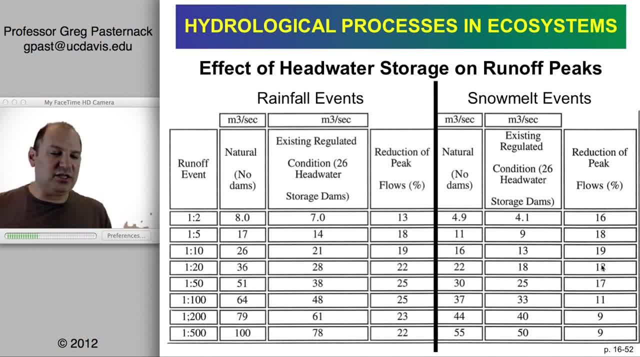 We see less of a fact and a little bit more like what I would expect, which is that a, you know, a range of nine to 19% reduction, with the largest events having the least benefit. Um, and the main explanation there is just that snow melt is not so much of an. 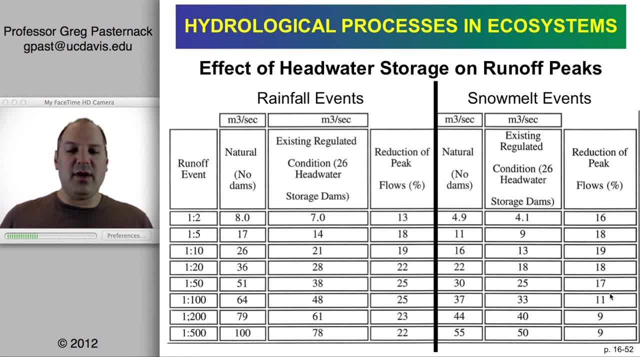 individual peak, but it's something that's happening through time And so, as a result, um, the model may not be as representative, um, and it's not. you know that a lot of things that are happening are not just related to the peak. 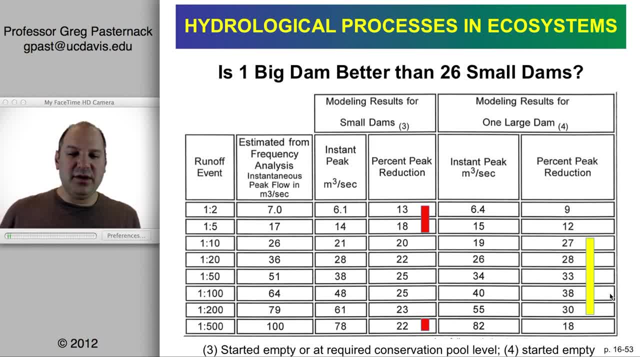 Is one dam better than 26 small dams? Well, when we do the head to head comparison, the percent reduction of small dams versus the percent reduction in for one large dam, um, where I've highlighted these like red bars, that's where the small dams have. 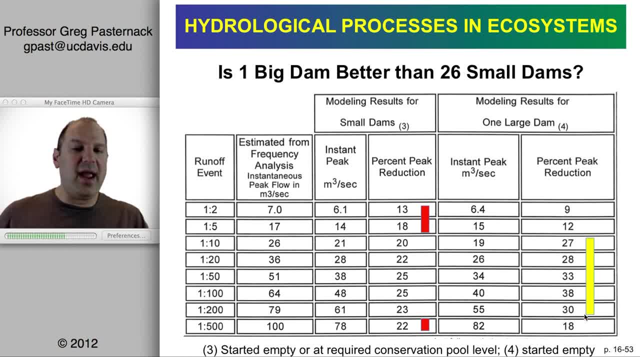 have performed the best. And then the yellow bar is the range of return interval events for which the large dam performed best. So the large dam, you know, performed about 30% better to 40% better If you compare the numbers compared to the small dams.